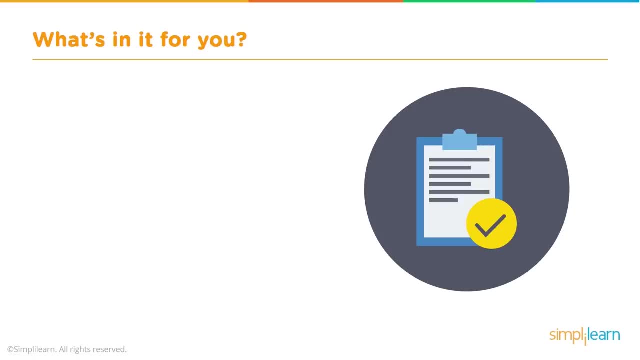 you don't have to worry, We will be brushing up the basics as well. So to start off with, let's have a look at the agenda here. First we'll look into our life without Machine Learning, Then we'll move into a life with Machine Learning. Then we'll try to understand what is Machine. 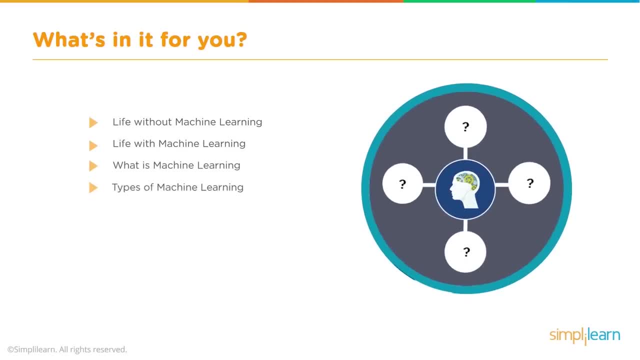 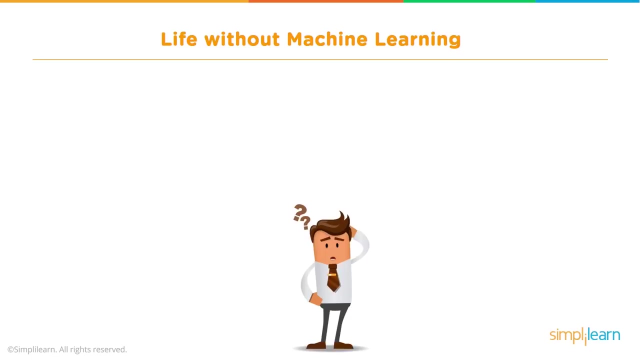 Learning actually. Then we'll look into the types of Machine Learning. We'll talk about the right Machine Learning solutions. Then we'll move into the different algorithms that Machine Learning has. Let's talk about our life without Machine Learning. For someone who doesn't know anything about machine learning or artificial intelligence, 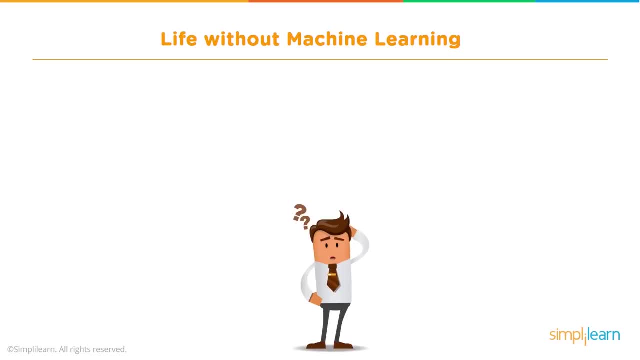 he or she might think that it is only being used in robots or machines and stuff, which is actually true, as portrayed by most of the sci-fi movies nowadays. But you wouldn't believe how much more machine learning is giving us, how much of it we are. 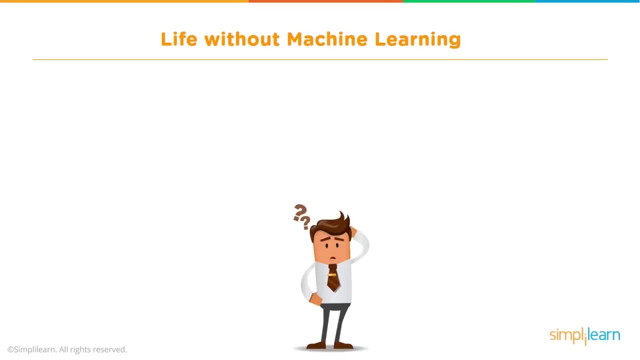 using in our daily lives. Let's say you need information on any random topic, say a computer, The first place you would check would definitely be Google. right, It would collect all the information on the word you search for and present it to you. 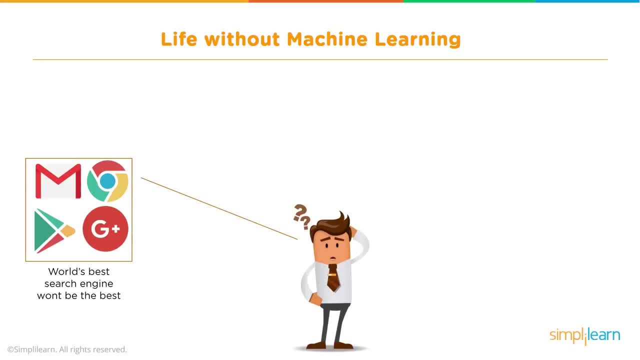 according to relevance. If there was no Google, you would have to do it in a very hard way, that is, by going through tens or hundreds of books and articles, even after which you won't find the answer. If we go back four to five years, facial recognition would be a thing only showed in movies like 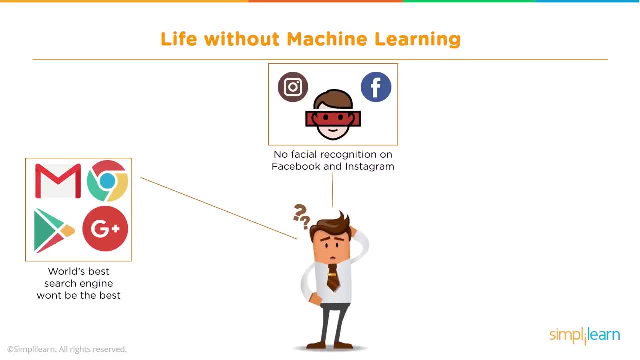 Mission Impossible or Terminator or any of the sci-fi movies you pick. But machine learning has made it possible for Facebook and Instagram to use this feature for your benefit. You don't have to go through the trouble of tagging every single person present in a picture that you have posted. 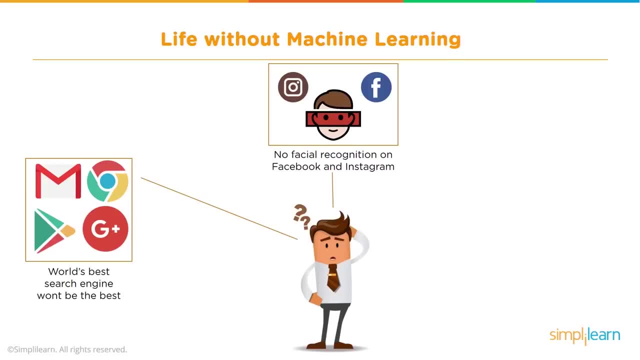 Facebook will automatically recognize the people in the photo and tag them for you. That saves a lot of time for you, doesn't it? Also, Siri, Cortana, Iris, all of them would not be there to help you if there was no machine. 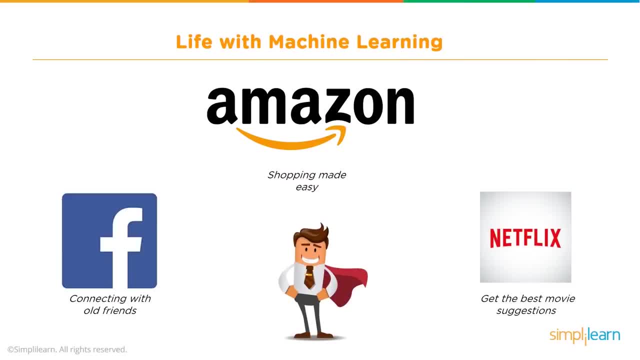 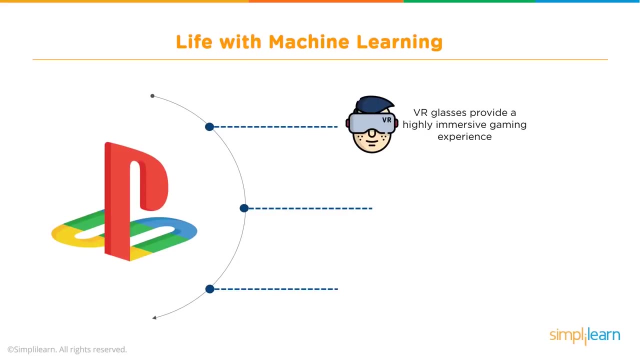 learning. Now that we know life would be a lot more difficult without machine learning, let's look into the things that are run by machine learning and we are used to. Let's start with the world of gaming. PS4's and Xboxes have introduced Virtual Reality Glasses, which brings a whole new level. 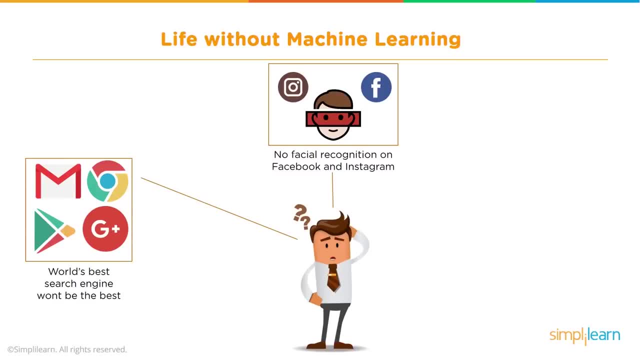 If we go back four to five years, facial recognition would be a thing only showed in movies like Mission Impossible or Terminator or any of the sci-fi movies you pick. But machine learning has made it possible for Facebook and Instagram to use this feature for your benefit. 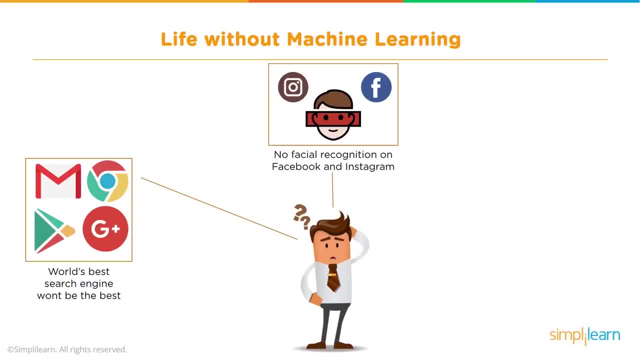 You don't have to go through the trouble of tagging every single person present in a picture that you have posted. Facebook will automatically recognize the people in the photo and tag them for you. That saves a lot of time for you, doesn't it? 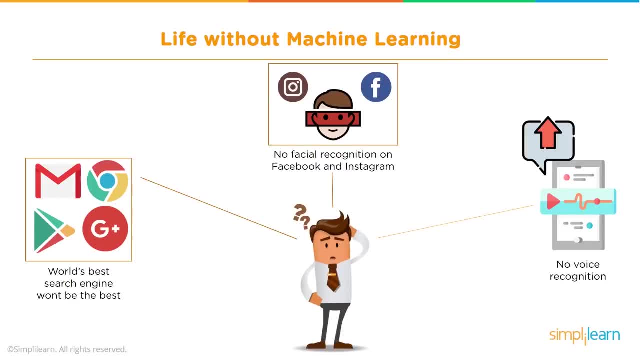 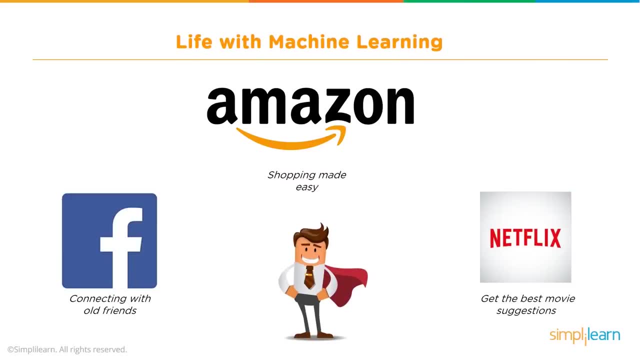 Also Siri, Cortana, Iris- all of them would not be there to help you if there was no machine learning. Now that we know life would be a lot more difficult without machine learning, let's look into the things that are run by machine learning and we are using. 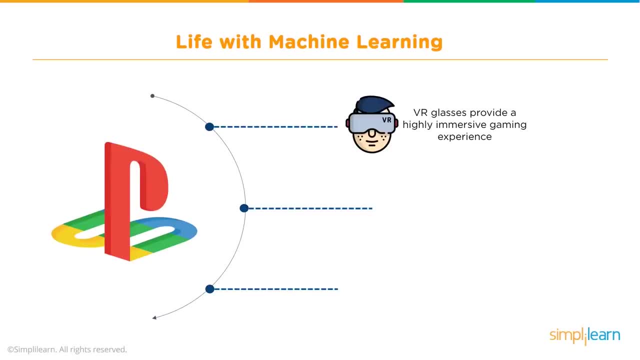 Let's enter the world of gaming. PS4's and Xbox's have introduced virtual reality glasses, which brings a whole new level of detail into gaming. Every time your head moves in real world, it replicates the movement in the virtual world, providing an excellent gaming experience. 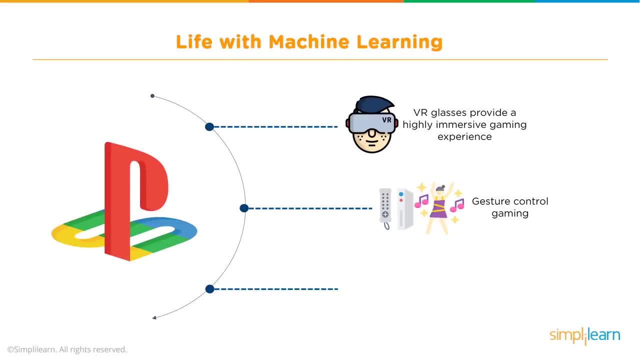 Then there is gesture control gaming, wherein machine learning tracks your body movement and makes a corresponding movement in the game. Finally, in the game FIFA, your opponent tends to match the movement of your body with the movement of your body. Finally, in the game FIFA, your opponent tends to match the movement of your body with the. 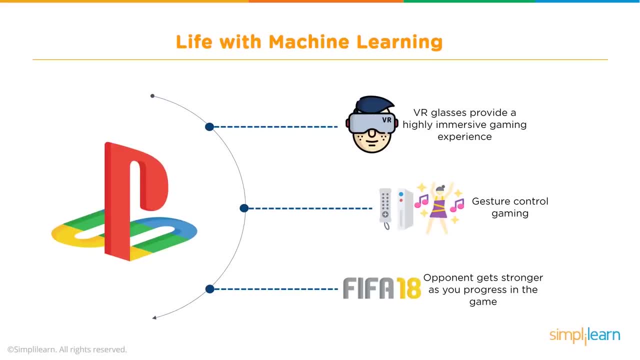 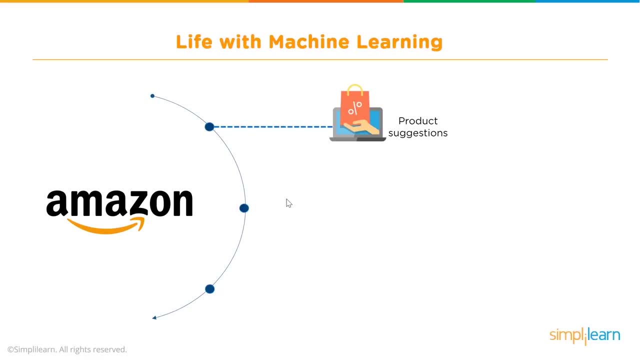 movement of your body tends to adapt based on the kind of strategy or gameplay you follow. That is again done by machine learning. I'm sure you must have shopped a lot from Amazon, So let's look into some of the places Amazon makes use of machine learning. 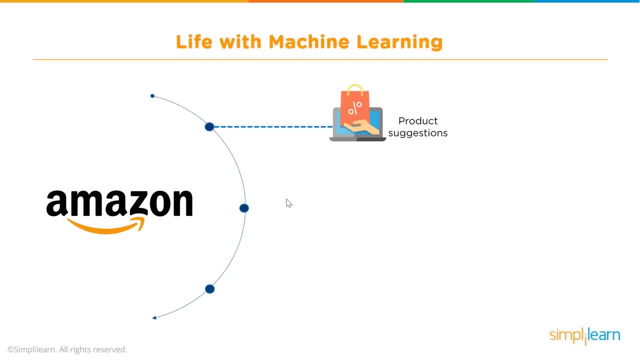 Let's say you buy a formal t-shirt on Amazon. As you buy it, it suggests you formal shoes, ties, blazers and apparels that go with what you have bought. That's the recommendation system powered by machine learning. again, The price on every product that you see on Amazon is varying every moment based on demand. 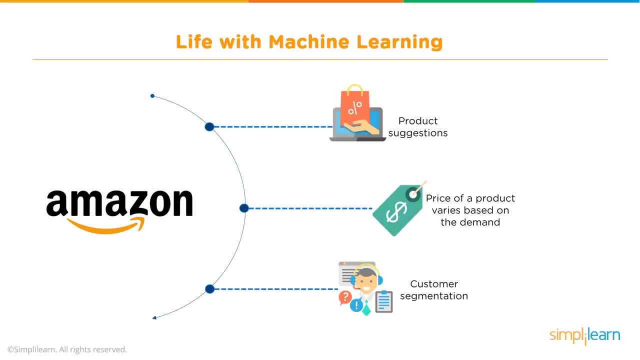 That's being done by machine learning algorithms. Then comes customer segmentation. Customer segmentation is one of the most crucial thing for all the e-commerce platforms. Machine learning helps them differentiate between customers based on what they buy, how frequent are they, and their reviews. 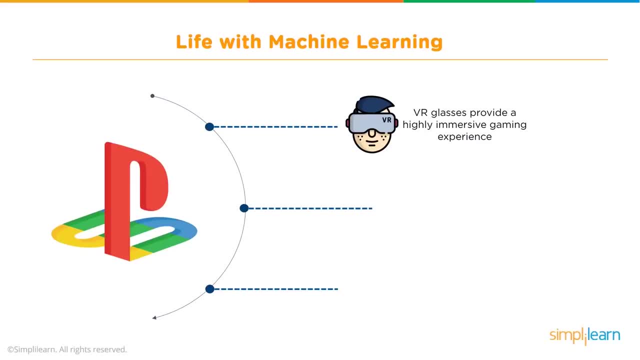 of detail into gaming. Every time your head moves in real world, it replicates the movement in the virtual world, providing an excellent gaming experience. Then there is Gesture Control Gaming, wherein machine learning tracks your body movement and makes a corresponding movement in the game. 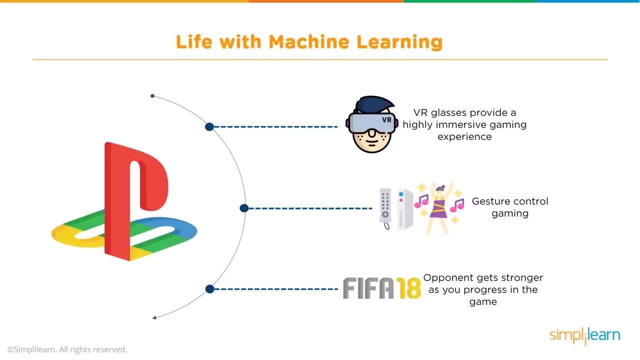 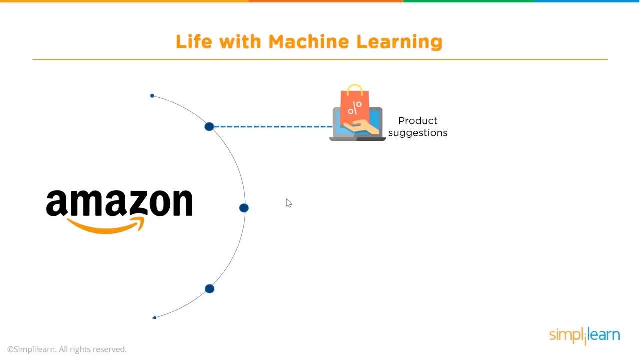 Finally, in the game FIFA…. Wait, tends to adapt based on the kind of strategy or gameplay you follow. That is again done by machine learning. I'm sure you must have shopped a lot from Amazon, So let's look into some of the places Amazon makes use of machine learning. 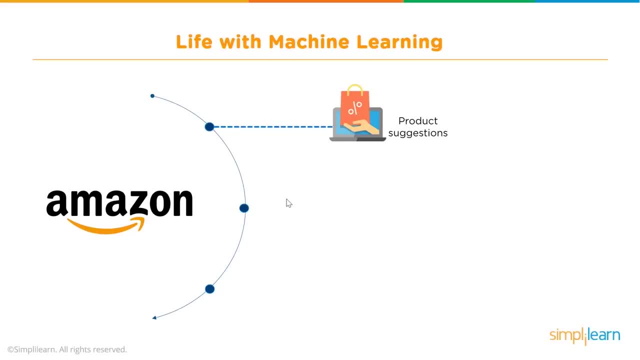 Let's say you buy a formal t-shirt on Amazon. Now, as you buy it, it suggests you formal shoes, ties, blazers and apparels that go with what you have bought. That's the recommendation system powered by machine learning. again, The price on every product that you see on Amazon is varying every moment, based on demand. 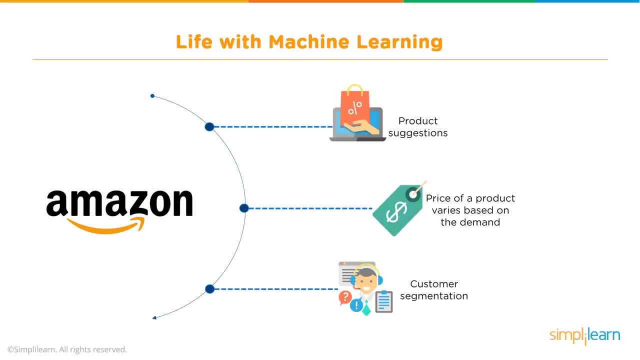 That's being done by machine learning algorithms. Then comes customer segmentation. Customer segmentation is one of the most crucial thing for all the e-commerce platforms. Machine learning helps them differentiate between customers based on what they buy, how frequent are they, and their reviews. 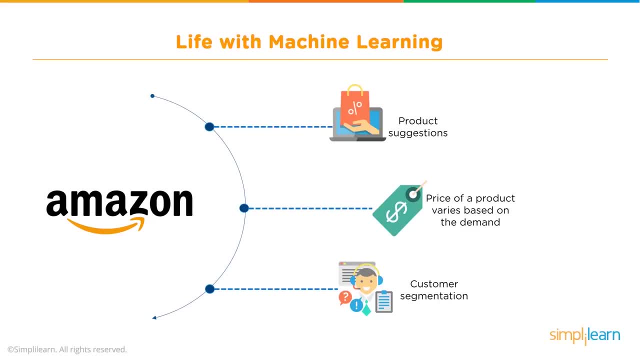 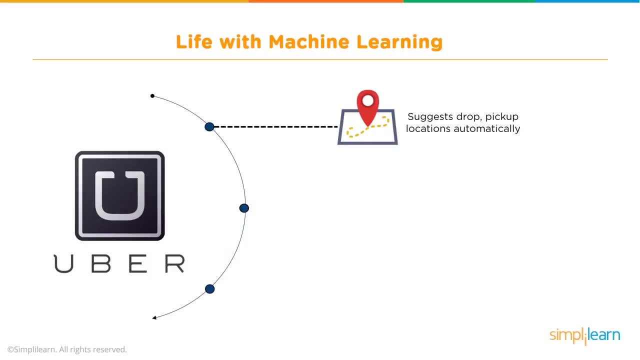 This helps the companies to make sure that their customers are taken care of and the needs are being fulfilled. Now let's talk about an app that you use on a daily basis to reach office on time. Yes, it's Uber cabs. Once you have travelled with Uber, you must have noticed that it suggests you the places 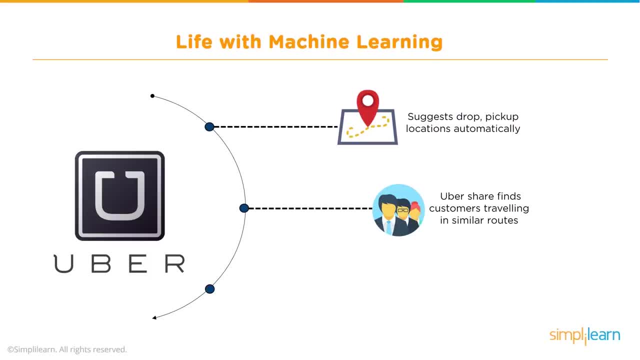 you might want to go, based on your previous journeys. When you are taking a share, how does the app make sure that the cab you get is travelled by the same route you want to travel in? There are so many factors, like the distance, the traffic, the ratings. 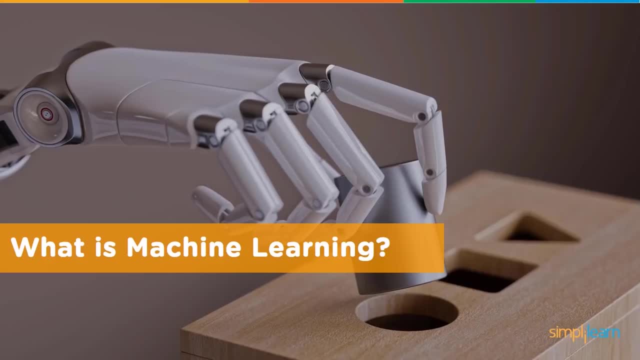 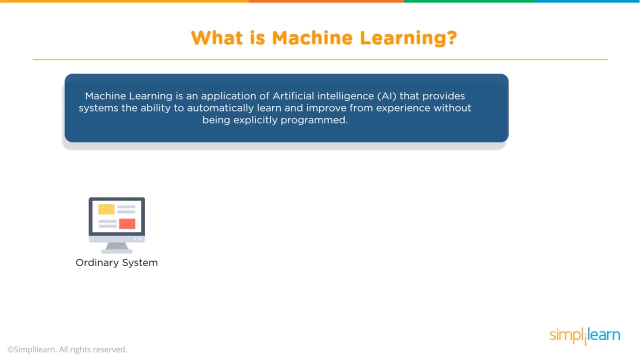 All of it is taken care of by machine learning. For the past 5 minutes, we have been talking about how machine learning is improving our lives, Where all it is being used. I have probably said machine learning a hundred times already. I think it's about time that I tell you what machine learning actually is. 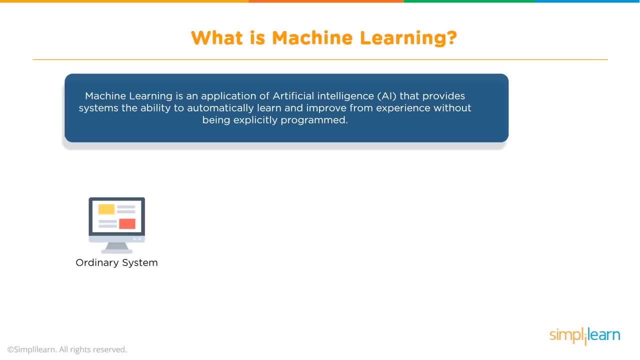 Let's take an ordinary system that you currently are using. It can't do much except from the basic operations that you already know about. Now let's add artificial intelligence or, for a layman's point of view, let's give the same machine the power to think on its own. 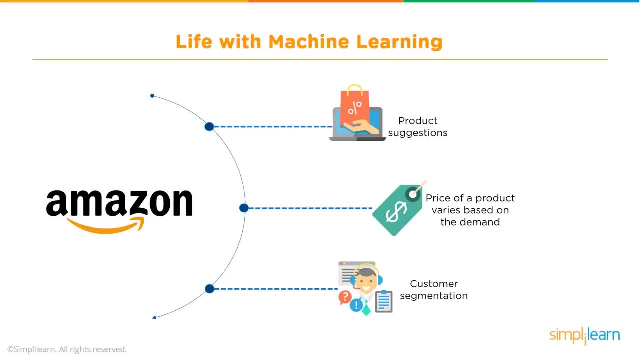 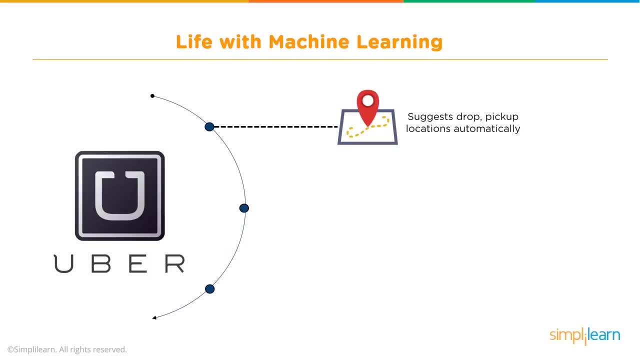 This helps the companies to make sure that their customers are taken care of and the needs are being fulfilled. Now let's talk about an app that you use on a daily basis to reach office on time. Yes, it's Uber cabs. Once you have travelled with Uber, you must have noticed that it suggests you the places 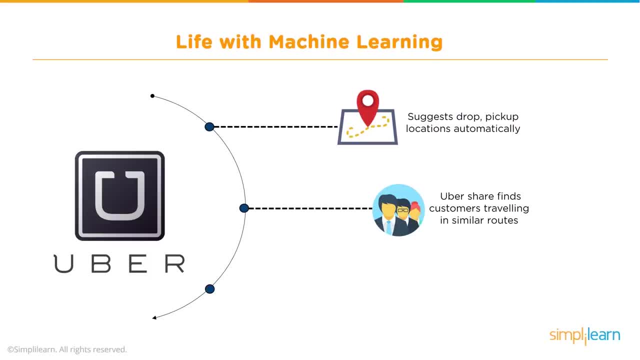 you might want to go, based on your previous journeys. When you are taking a share, how does the app make sure that the cab you get is travelled by the same route you want to travel in? There are so many factors, like the distance, the traffic, the ratings. 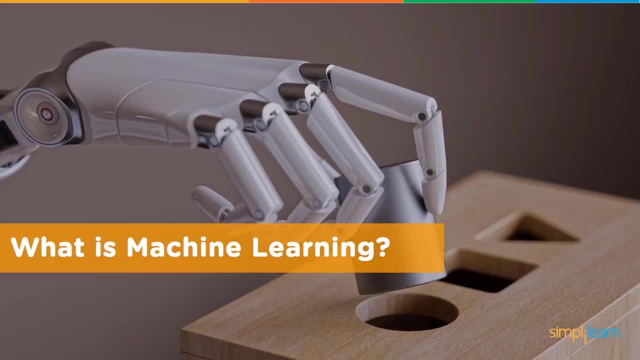 All of it is taken care of by machine learning. For the past five years, I've been using Uber. I've been using Uber. For the past five minutes, we have been talking about how machine learning is improving our lives, where all it is being used. 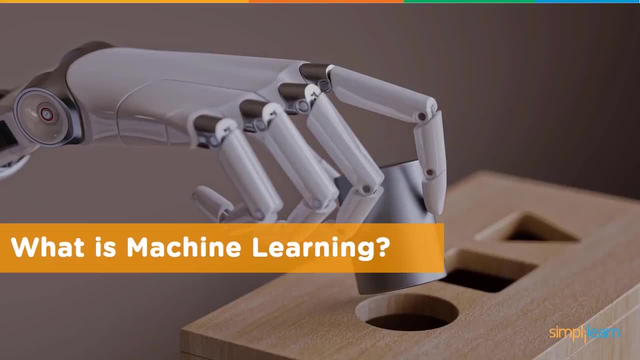 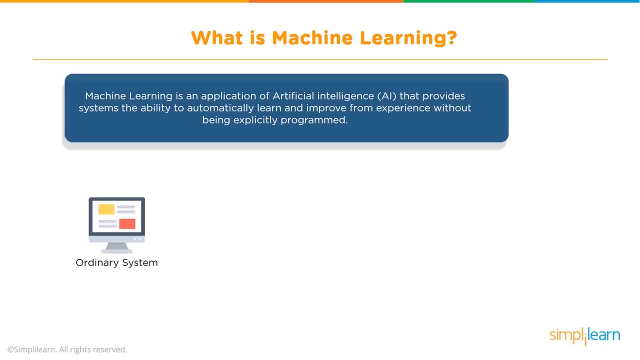 I have probably said machine learning a hundred times already. I think it's about time that I tell you what machine learning actually is. Let's take an ordinary system that you currently are using. It can't do much except from the basic operations that you already know about. 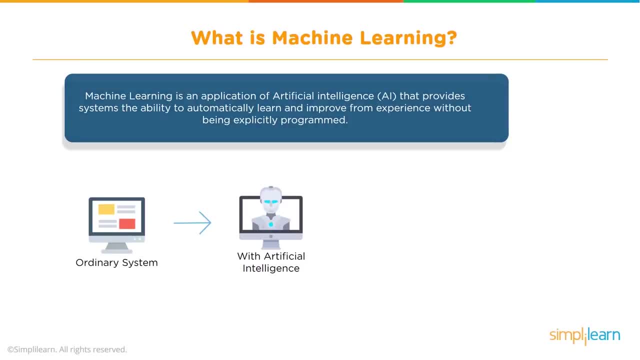 Now let's add artificial intelligence or, for a layman's point of view, let's give the same machine the power to think on its own. It's what machine learning basically is. It's an application of artificial intelligence that provides systems the ability to learn. 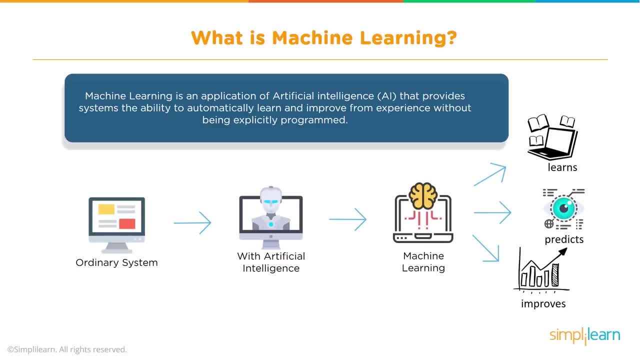 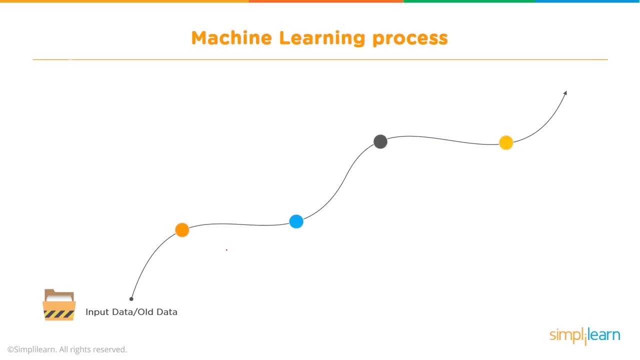 on their own and improve from experience without being programmed externally. So if your computer had machine learning, it may be able to play the difficult parts of a game for you or probably solve a complicated mathematical equation for you. That could be really helpful. Let's dive in a little deeper and see how machine learning works. 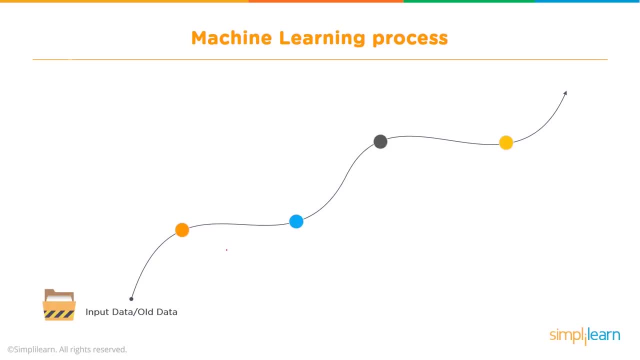 Let's say you provide a system with the input data that carries the photos of various kinds of fruits. Now you want the system to figure out what are the different fruits and group them accordingly. So what the system does? it analyzes the input data. 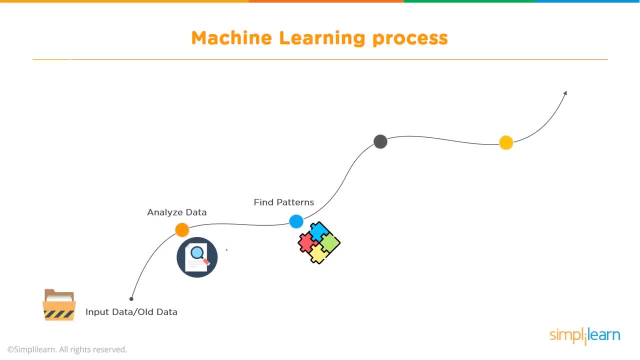 Then it tries to find patterns- patterns like shapes, size and color. Based on these patterns, the system will try to predict the different types of fruit and segregate them. Finally, it keeps track of all such decisions it took in the process to make sure it's. 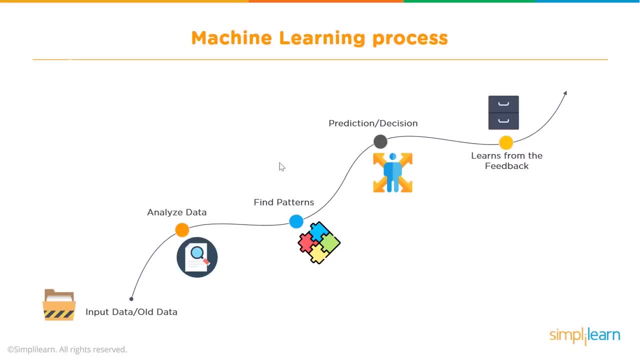 learning. The next time you ask the same system to predict and segregate the different types of fruits, it won't have to go through the entire process again. That's how machine learning works. Now let's look into the types of machine learning. 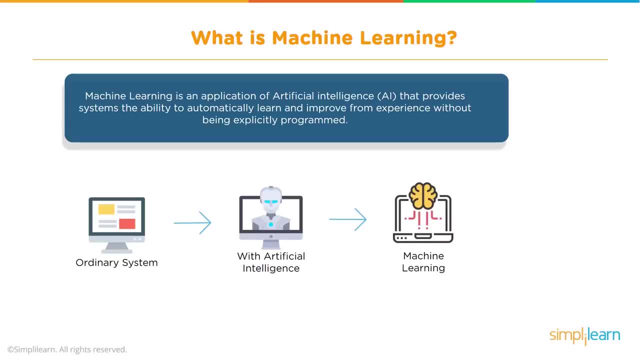 That is what machine learning basically is. It's an application of artificial intelligence that provides systems the ability to learn on their own and improve from experience without being programmed externally. So if your computer had machine learning, it may be able to play the difficult parts. 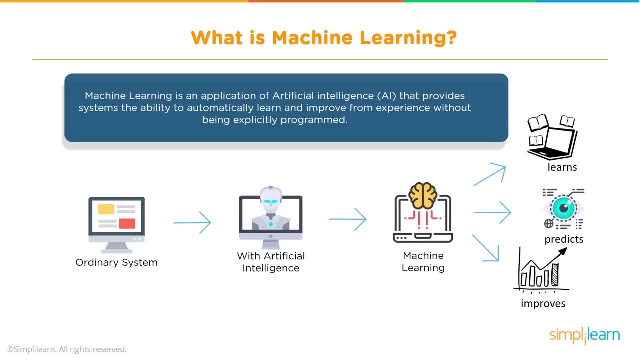 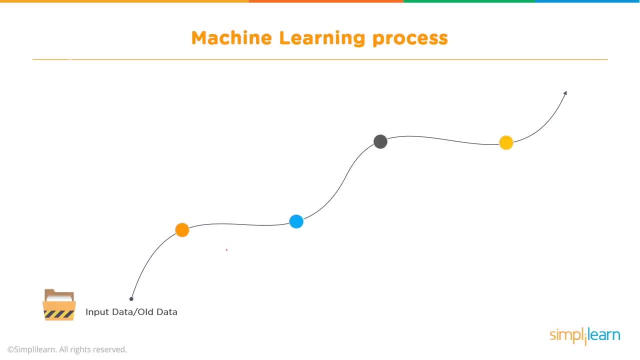 of a game for you or probably solve a complicated mathematical equation for you. That could be really helpful. Let's dive in a little deeper and see how machine learning works. Let's say you provide a system with the input data that carries the 14-digit number. 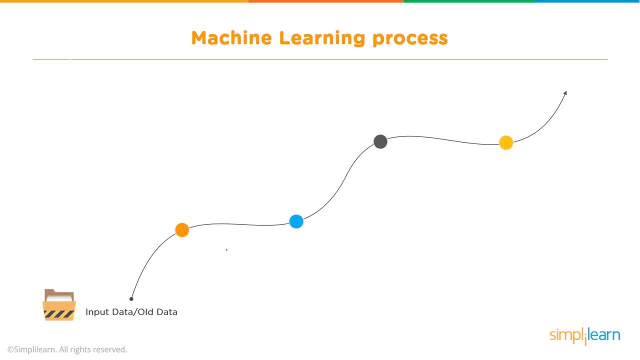 Let's see how machine learning works. Let's say you provide a system with the photos of various kinds of fruits. Now you want the system to figure out what are the different fruits and group them accordingly. So what the system does? it analyzes the input data. 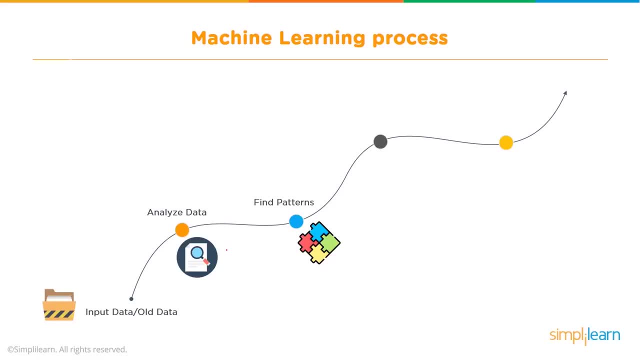 Then it tries to find patterns- patterns like shapes, size and color. Based on these patterns, the system will try to predict the different types of fruit and segregate them. Finally, it keeps track of all such decisions it took in the process to make sure it's learning. 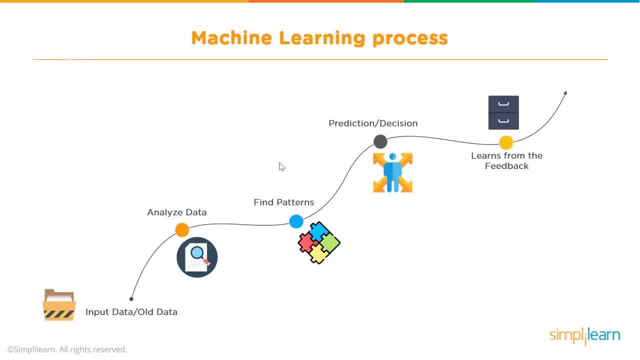 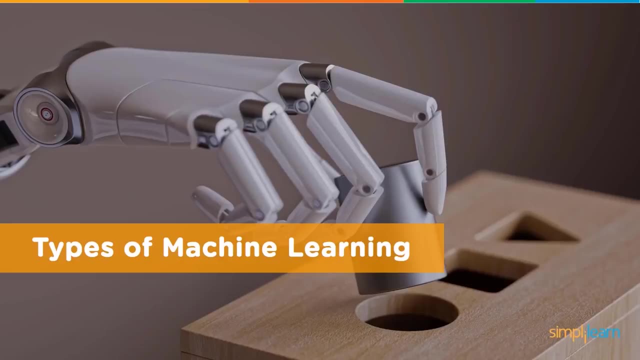 So if you have a machine learning system to predict and segregate the different types of fruits, it won't have to go through the entire process again. That's how machine learning works. Now let's look into the types of machine learning. Machine learning is primarily of three types. 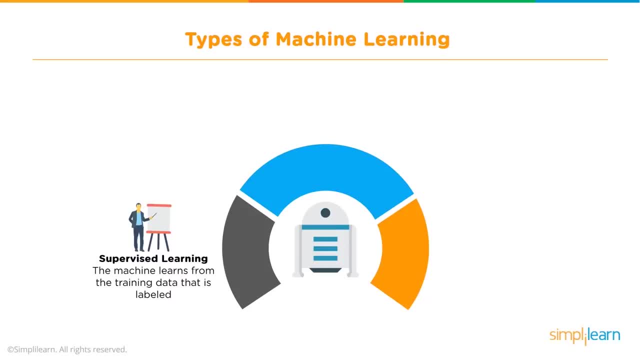 First one is supervised machine learning. As the name suggests, you have to supervise your machine learning while you train it to work on its own. It requires labeled training data. Next up is unsupervised learning, wherein there will be training data But it won't be labeled. 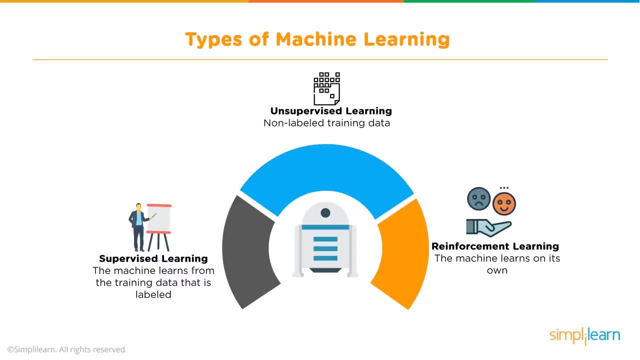 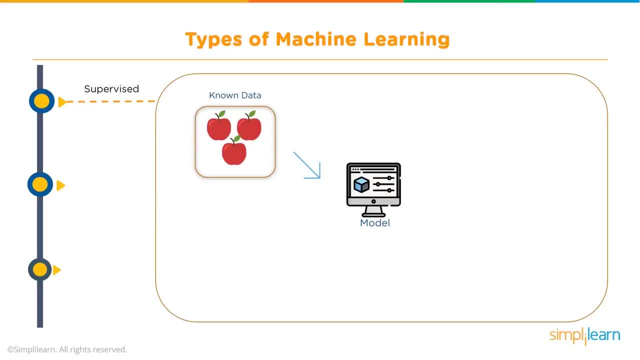 Finally, there is reinforcement learning, wherein the system learns on its own. Let's talk about all these types in detail. Let's try to understand how supervised learning works. Look at the pictures very, very carefully. The monitor depicts the model or the system that we are going to train. 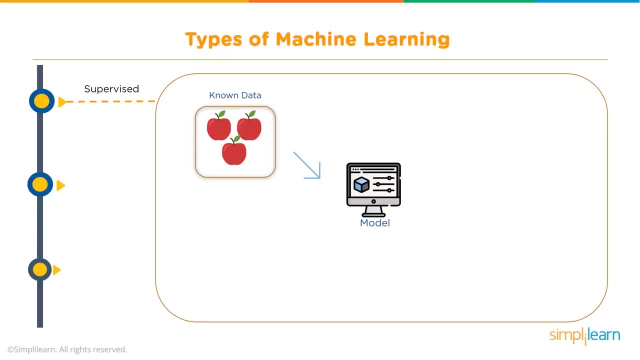 This is how the training is done. We provide a data set that contains pictures of a kind of a fruit, say an apple. Then we provide another data set which lets the model learn. The model will know that these pictures were that of a fruit called apple. 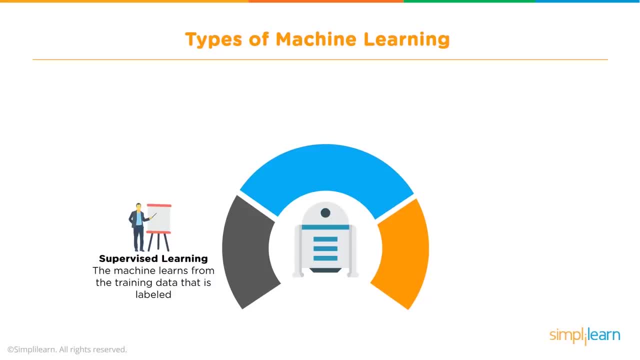 Machine learning is primarily of three types. First one is supervised machine learning. As the name suggests, you have to supervise your machine learning while you train it to work on its own. It requires labeled training data. Next up is unsupervised learning, wherein there will be training data but it won't be labeled. 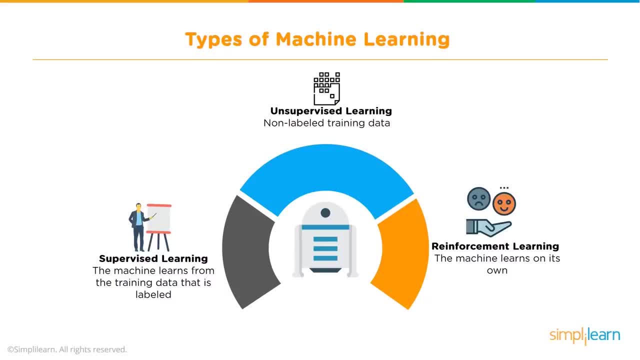 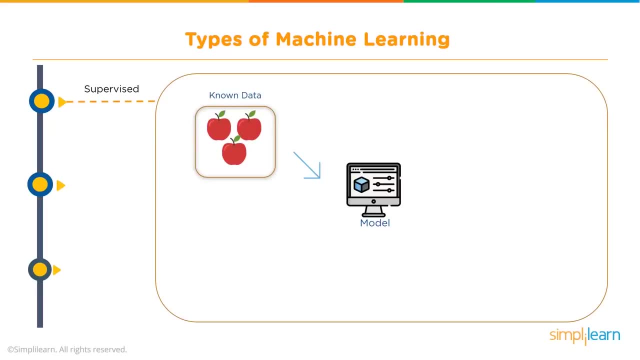 Finally, there is reinforcement learning, wherein the system learns on its own. Let's talk about all these types in detail. Let's try to understand how supervised learning works. Look at the pictures very, very carefully. The monitor depicts the model or the system that we are going to train. 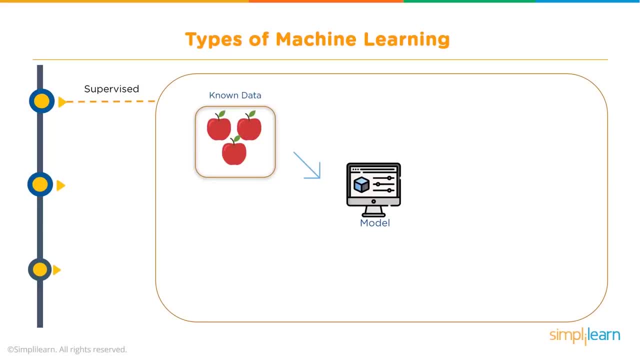 This is how the training is done. We provide a dataset that contains pictures of a kind of a fruit, say an apple. Then we provide another dataset which lets the model know that these pictures were the that of a fruit called apple. This ends the training phase. 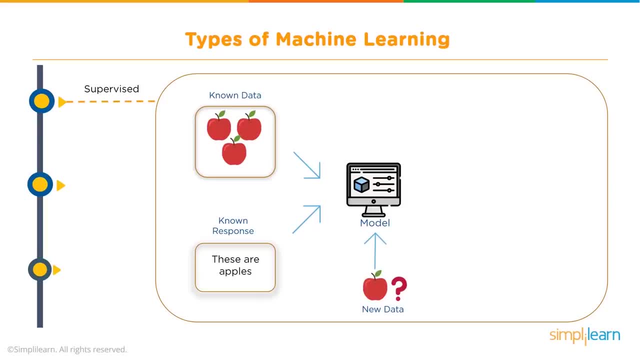 Now what we will do is we provide a new set of data which only contains pictures of apple. Now here comes the fun part: The system can actually tell you what fruit it is, And it will remember this and apply this knowledge in future as well. 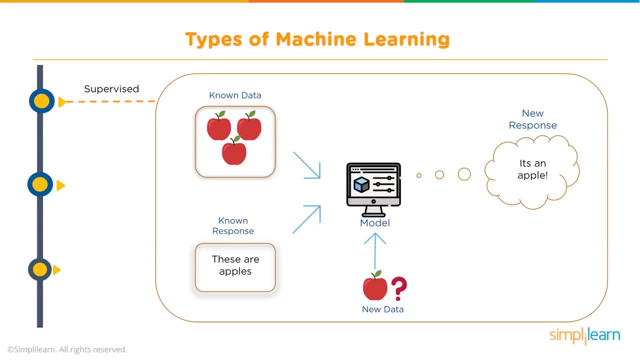 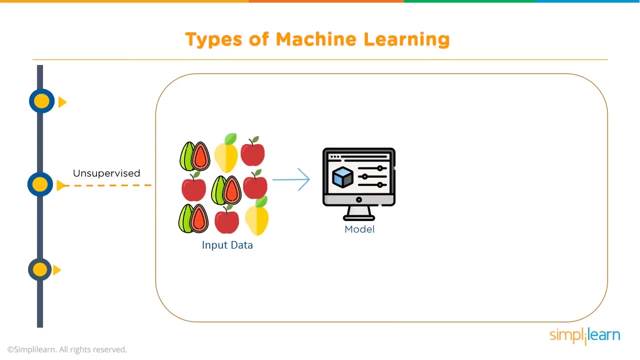 That's how supervised learning works. You are training the model to do a certain kind of an operation on its own. This kind of a model is generally used into filtering spam mails from your website. This is how supervised learning works 鈰. So let's move on to unsupervised learning. now let's say we have a dataset which is 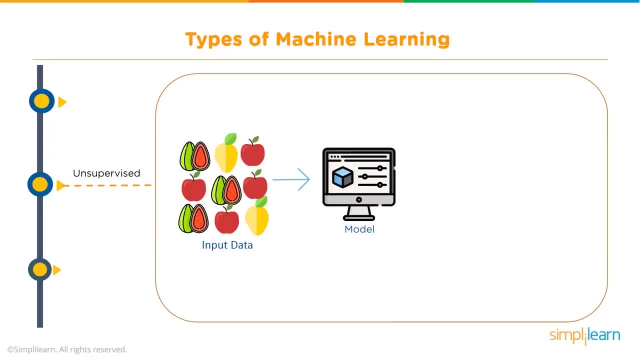 cluttered. In this case, we have a collection of pictures of different fruits. We feed this data to the model and the model analyzes the data to figure out patterns in it. In the end, it categorizes the photos into three types, as you can see in the image based. 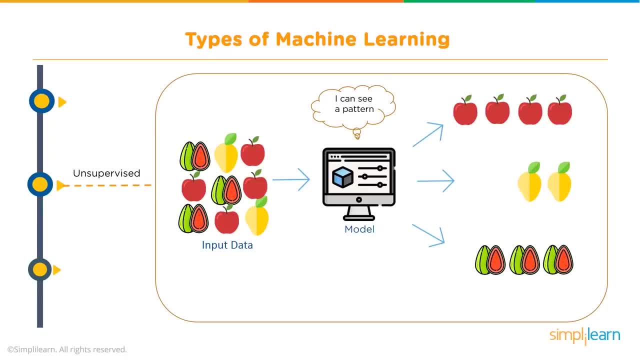 on their similarities. So you provide the data to the system and let the system do the rest of the work. Simple, isn't it? This kind of a model is used by Flipkart to figure out the products that are well suited for you. 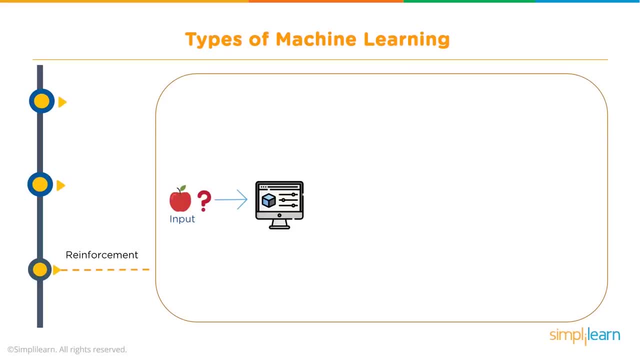 Honestly speaking, this is my favorite type of machine learning out of all the three, and this type has been widely shown in most of the sci-fi movies lately. Let's find out how it works. Imagine a newborn baby. You put a burning candle in front of the baby. 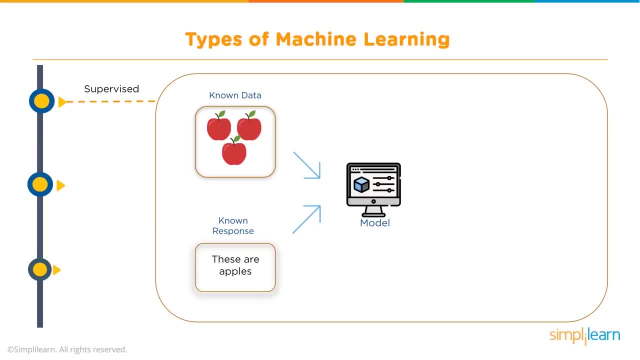 This ends the training phase. Now what we will do is we provide a new set of data which only contains pictures of apple. Now here comes the fun part: The system can actually tell you what fruit it is, And it will remember this and apply this knowledge in future as well. 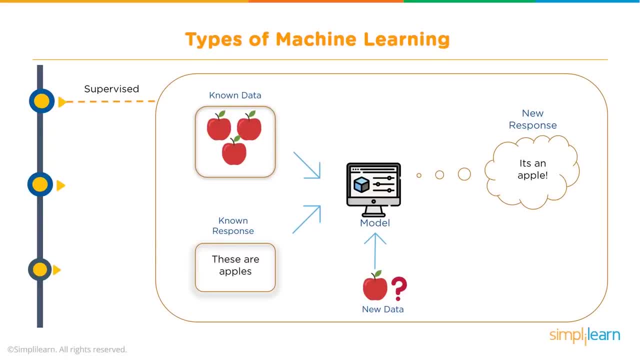 That's how supervised learning works. You are training the model to do a certain kind of an operation on its own. This kind of a model is generally used to train the model to do a certain kind of an operation on its own. This kind of a model is generally used into filtering spam mails from your email accounts. 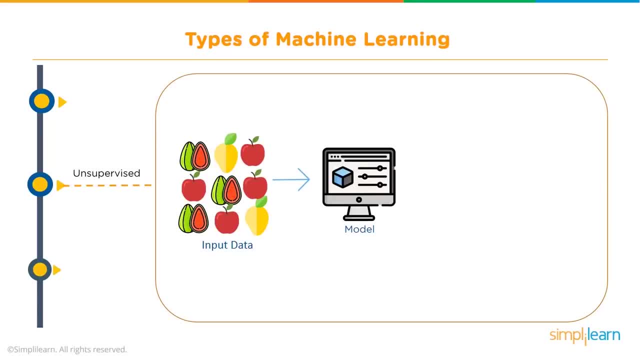 as well. Yes, surprise, aren't you? So let's move on to unsupervised learning. now Let's say we have a data set which is cluttered, In this case we have a collection of pictures of different fruits. We feed this data to the model and the model analyzes the data to figure out patterns in 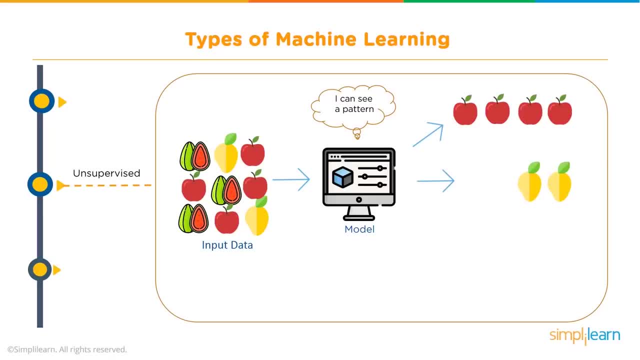 it. In the end, it categorizes the photos into three types, as you can see in the image, based on their similarities. So you provide the data to the system and let the system do its job. Simple, isn't it? This kind of a model is used by Flipkart to figure out the products that are well suited. 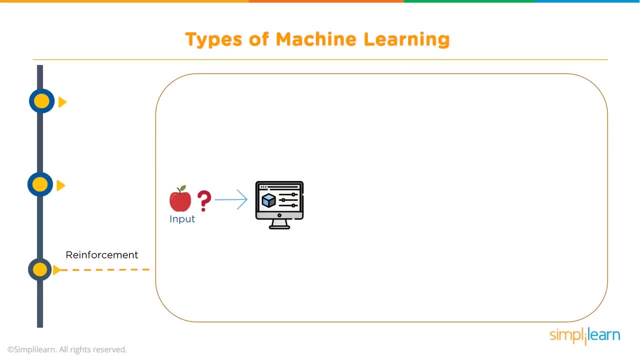 for you. Honestly speaking, this is my favorite type of machine learning out of all the three, And this type has been widely shown in most of the sci-fi movies lately. Let's find out how it works. Imagine a newborn baby. You put a burning candle in front of the baby. 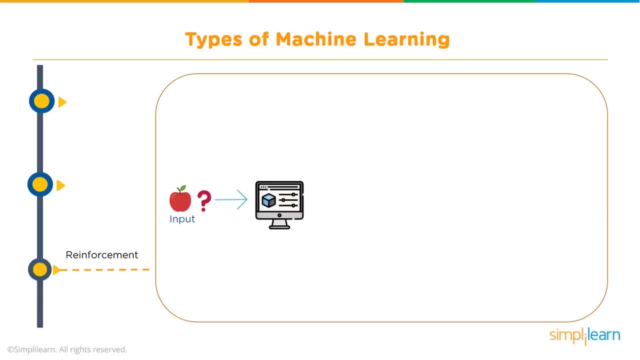 The baby does not know that if it touches the flame its fingers might get burned, So it does that for you. You put a burning candle in front of the baby, It does that anyway and gets hurt. The next time you put that candle in front of the baby it will remember what happened. 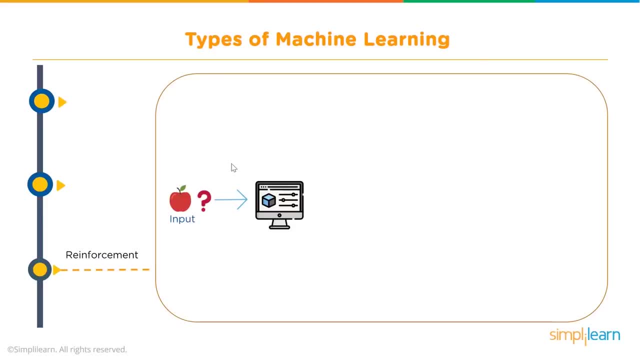 the last time and would not repeat what it did. That's exactly how reinforcement learning works. We provide the machine with a dataset wherein we ask it to identify a particular kind of a fruit, in this case an apple. So what it does as a response, it tells us that it's a mango. 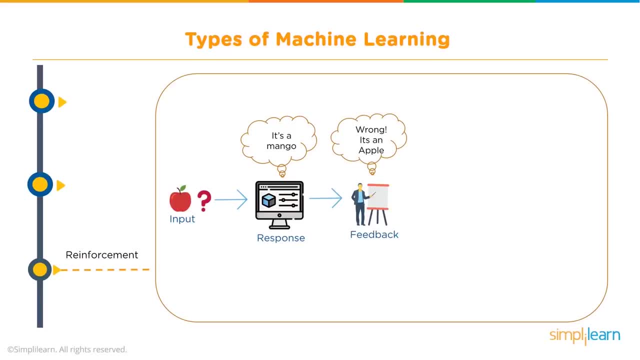 But, as we all know, it's a completely wrong answer. So, as a feedback, we tell the system that it's wrong. It's not a mango, It's an apple. What it does, it learns from the feedback and keeps that in mind. 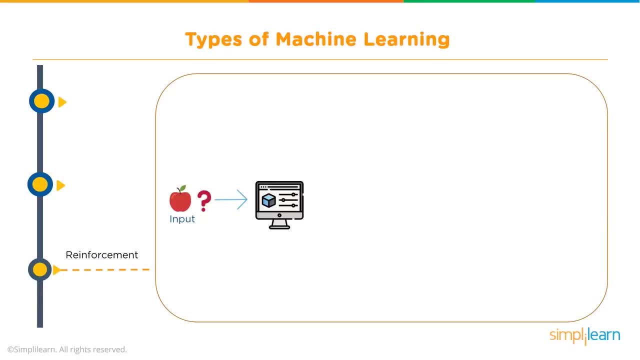 The baby does not know that if it touches the flame its fingers might get burned, So it does that anyway and gets hurt. The next time you put that candle in front of the baby it will remember what happened the last time and would not repeat what it did. 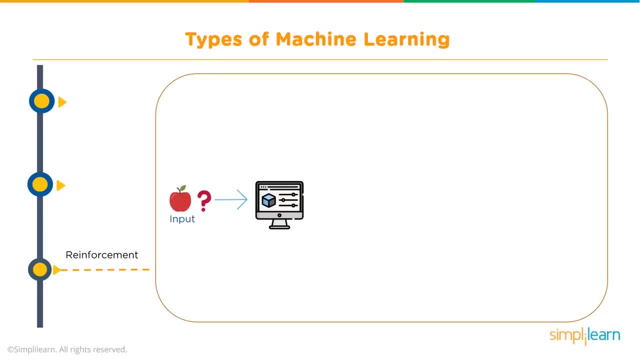 That's exactly how reinforcement learning works. We provide the machine with a data set wherein we ask it to identify a particular kind of a fruit, in this case an apple. So what it does as a response, it tells us that it's a mango. 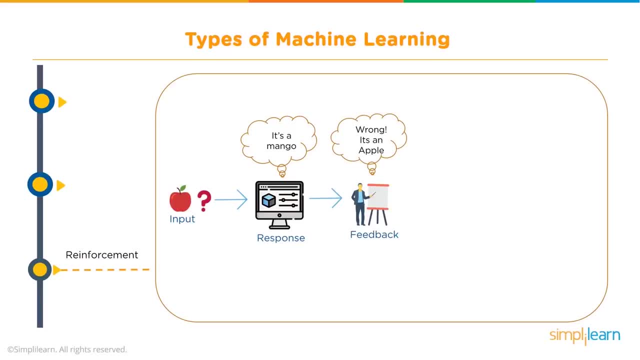 But, as we all know, it's a completely wrong answer. So, as a feedback, we tell the system that it's wrong. It's not a mango, It's an apple. What it does, it learns from the feedback and keeps that in mind. 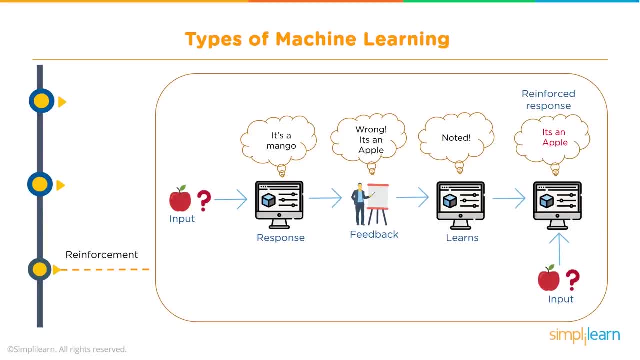 When, the next time, when we ask a same question, it gives us the right answer, It is able to tell us that it's actually an apple. That is a reinforced response. So that's how reinforcement learning works: It learns from its mistakes and experiences. 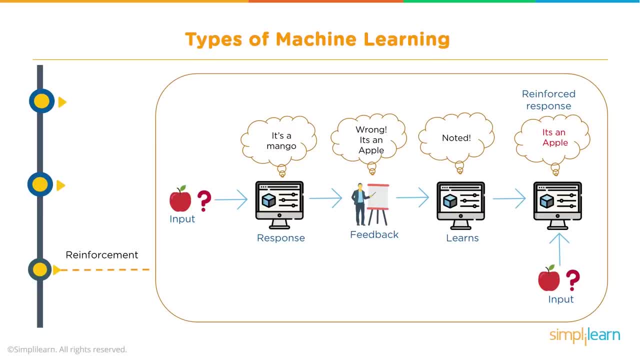 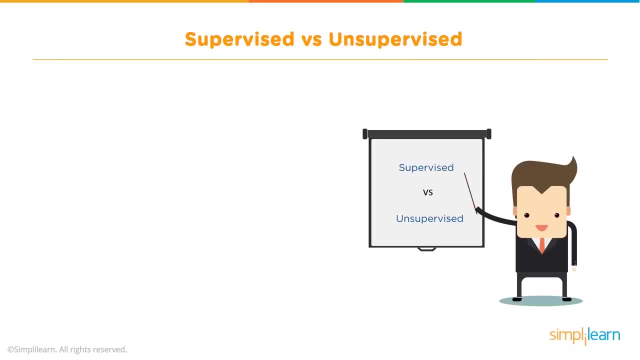 This model is used in games like Prince of Persia or Assassin's Creed or FIFA, wherein the level of difficulty increases as you get better with the games. Just to make it more clear for you, Let's look at a comparison between supervised and unsupervised learning. 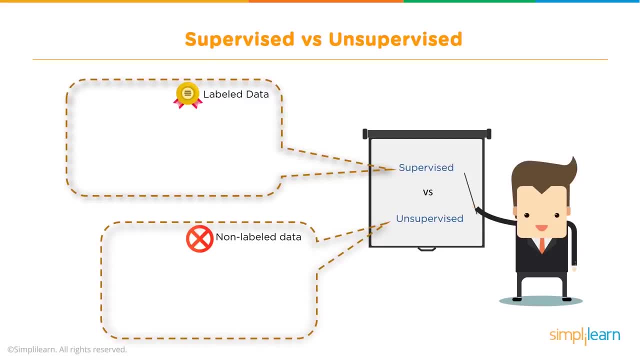 Firstly, the data involved in case of supervised learning is labeled. As we mentioned in the examples previously, we provide the system with a photo of an apple and let the system know that this is actually an apple. That is called labeled data. So the system learns from the labeled data and makes future predictions. 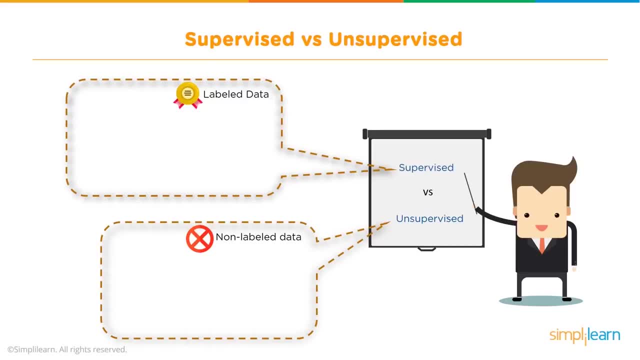 Now, unsupervised learning does not require any kind of labeled data, because its work is to look for patterns in the input data and organize it. The next point is that you get a feedback. in case of supervised learning, That is, once you get the output. the system tends to remember that and uses it for the next operation. 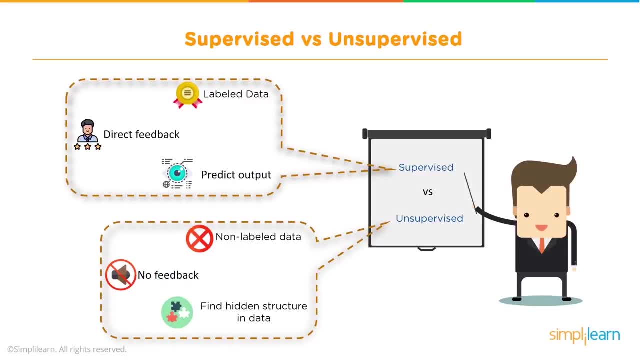 That does not happen for unsupervised learning. And the last point is that supervised learning is mostly used to predict data, Whereas unsupervised learning is used to find out hidden patterns or structures in data. I think this would have made a lot of things clear for you. 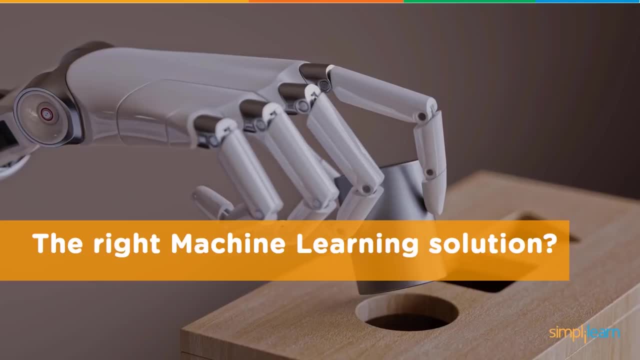 So let's move on to the next point. So let's move on to the next point. Now let's talk about a question that everyone needs to answer before building a machine learning model: What kind of a machine learning solution should we use? 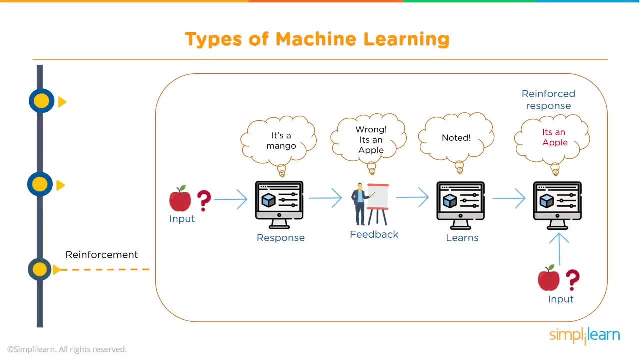 When, the next time, when we ask a same question, it gives us the right answer, It is able to tell us that it's actually an apple. That is a reinforced response. So that's how reinforcement learning works: It learns from its mistakes and experiences. 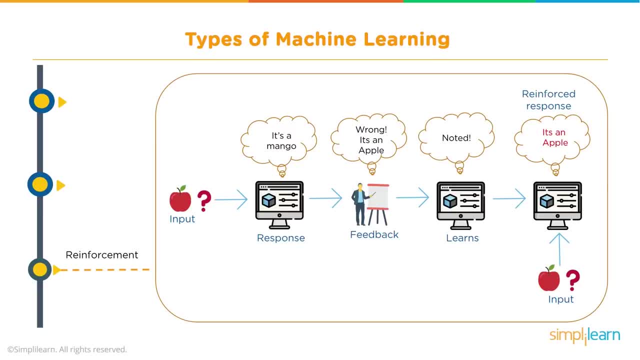 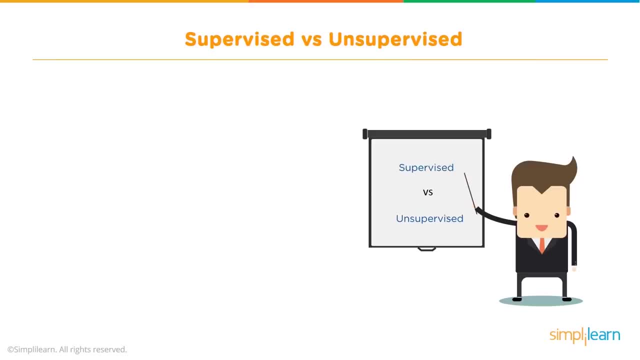 This model is used in games like Prince of Persia or Assassin's Creed or FIFA, wherein the level of difficulty increases as you get better with the games. Just a reminder, Just to make it more clear for you, let's look at a comparison between supervised and. 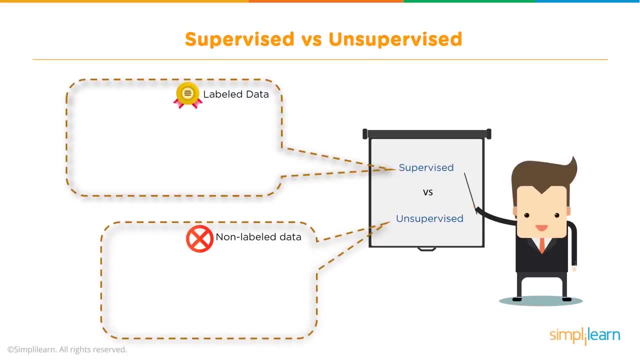 unsupervised learning. Firstly, the data involved in case of supervised learning is labelled. As we mentioned in the examples previously, we provide the system with a photo of an apple and let the system know that this is actually an apple. That is called labelled data. 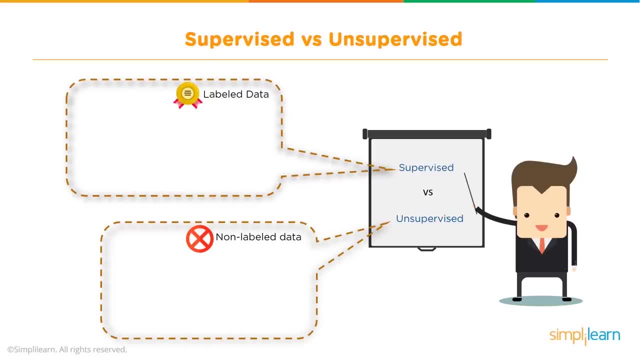 So the system learns from the labelled data and makes future predictions. Now, unsupervised learning does not require any kind of labelled data, Because its work is to look for patterns in the input data and organise it. The next point is that you get a feedback in case of supervised learning. 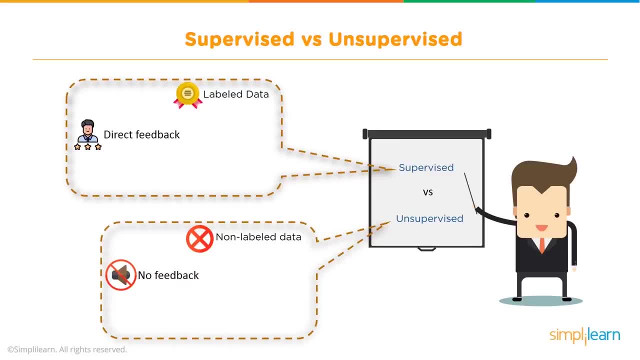 That is, once you get the output, the system tends to remember that and uses it for the next operation. That does not happen for unsupervised learning. And the last point is that supervised learning is mostly used to predict data, whereas unsupervised. 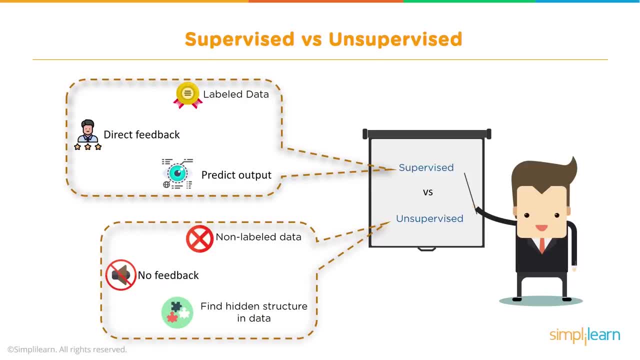 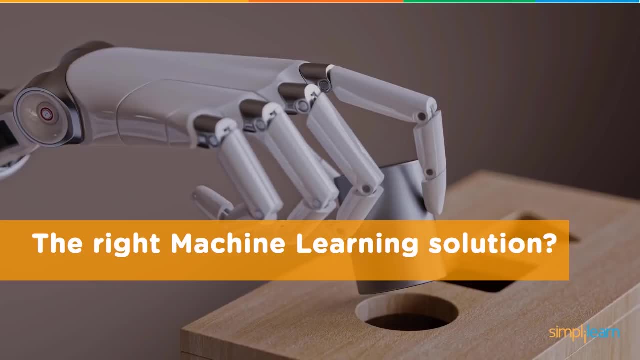 learning is used to find out hidden patterns or structures in data. I think This would have made a lot of things clear for you regarding supervised and unsupervised learning. Now let's talk about a question that everyone needs to answer before building a machine. 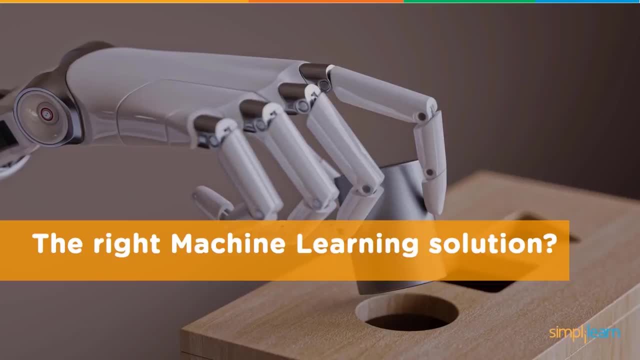 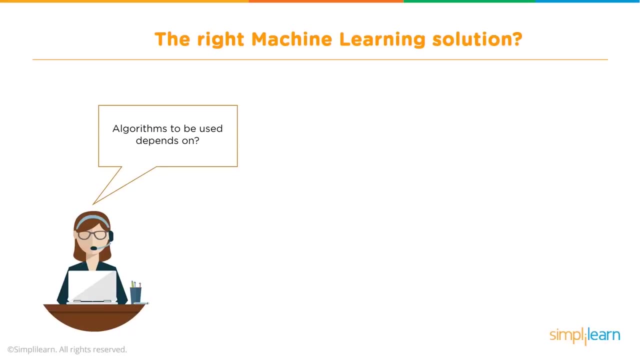 learning model. What kind of a machine learning solution should we use? Yes, you should be very careful with selecting the right kind of solution for your model, Because if you don't, you might end up losing a lot of time, energy and processing cost. 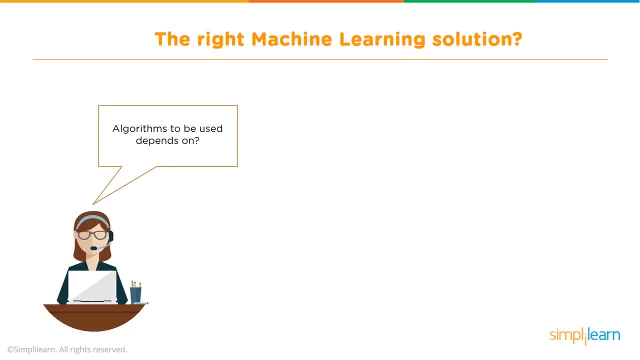 I won't be naming the actual solutions because you guys aren't familiar with them yet, So we will be looking at it based on the results. So let's look into the factors that might help us select the right kind of machine learning solution. First factor is the problem statement. describes the kind of model you will be building, or 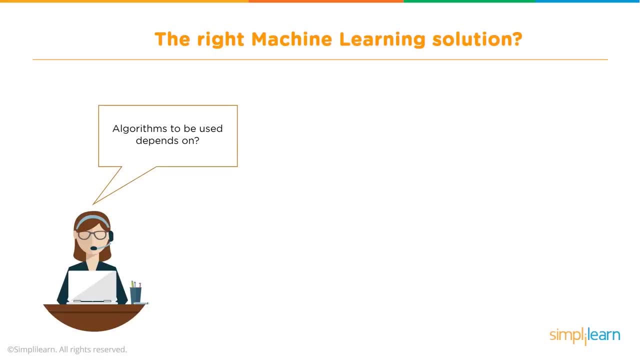 Yes, you should be very careful with selecting the right kind of solution for your model, Because if you don't, you might end up losing a lot of time, energy and processing cost. I won't be naming the actual solutions because you guys aren't familiar with them yet. 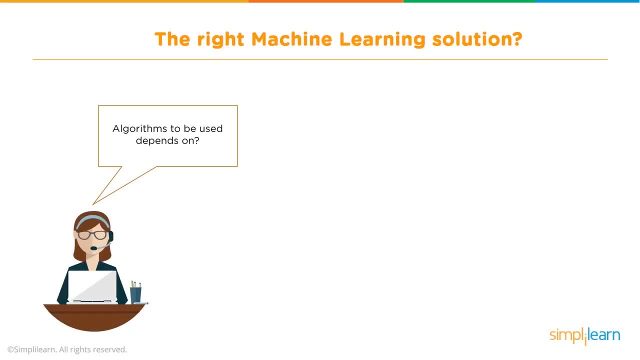 So we will be looking at it, based on supervised, unsupervised and unsupervised learning. So let's look into the factors that might help us select the right kind of machine learning solution. First factor is the problem statement describes the kind of model you will be building or, as the name suggests, it tells you what the problem is. 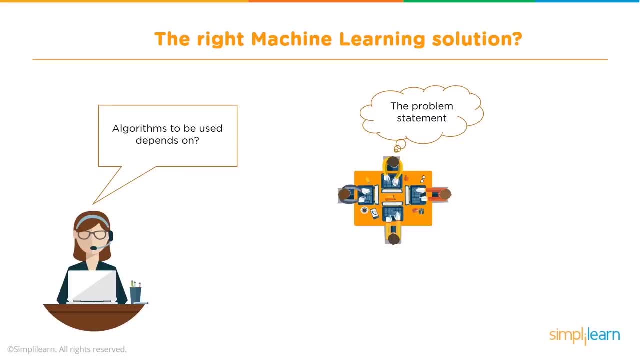 For example, let's say the problem is to predict the future stock market prices. So for anyone who is new to machine learning would have trouble figuring out the right solution. But with time and practice you will understand that for a problem statement like this, a solution based on supervised learning would work the best, for obvious reasons. 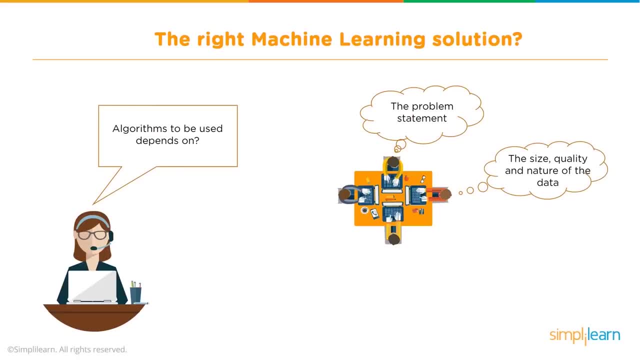 Then comes the size, quality and nature of the data. If the data is cluttered, you go for unsupervised. If the data is very large and categorical, we normally go for supervised learning solutions. Finally, we choose a solution based on their complexity. 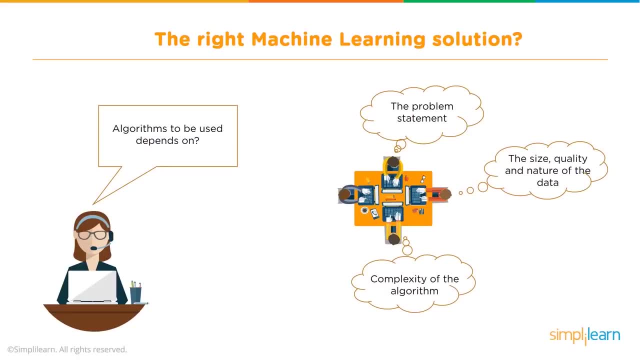 As for the problem statement wherein we predict the stock market prices, it can also be solved by using reinforcement learning, But the problem statement says that the problem statement should be based on the complexity of the solution. But that would be very, very difficult and time-consuming, unlike supervised learning. 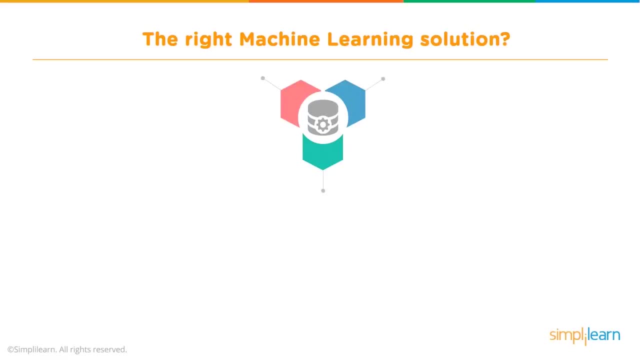 Algorithms are not types of machine learning. In the most simplest language, they are methods of solving a particular problem. So the first kind of method is classification, which falls under supervised learning. Classification is used when the output you are looking for is a yes or a no, or in the form A or B, or true or false. 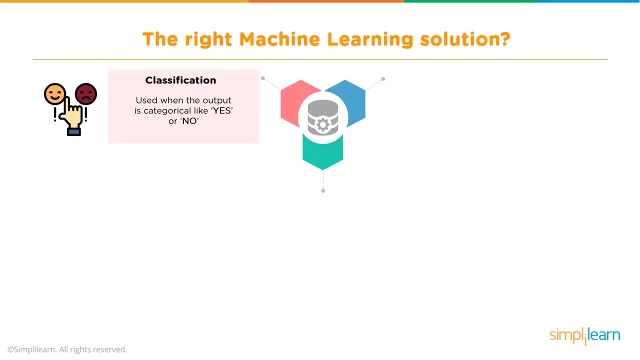 Like if a shopkeeper wants to predict if a particular customer will come back to his shop or not, he will use a classification algorithm. The algorithms that fall under classification are decision tree knife base, random forest logistic regression and KNN. 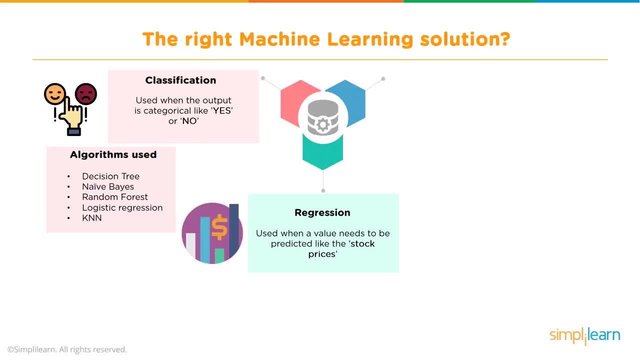 The next kind is regression. This kind of a method is used when the predicted data is numerical in nature, Like if the shopkeeper wants to predict the price of a product based on its demand. it would go for regression. The last method is clustering. 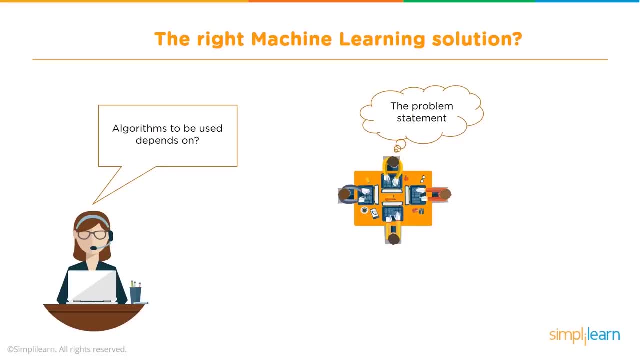 as the name suggests, it tells you what the problem is. For example, let's say the problem is to predict the future stock market prices. So for anyone who is new to machine learning would have trouble figuring out the right solution. But with time and practice you will understand the problem. 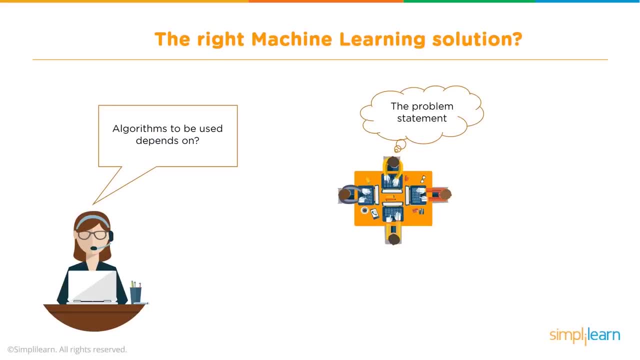 So let's look into the factors that might help us select the right kind of machine learning solution. Let's first understand that for a problem statement like this, solution based on supervised learning would work the best, for obvious reasons. Then comes the size, quality and nature of the data. 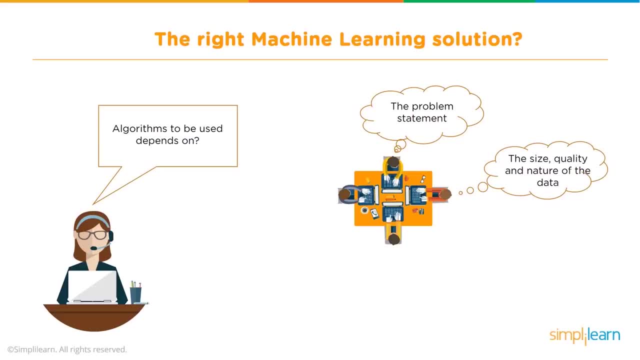 If the data is cluttered, you go for unsupervised. If the data is very large and categorical, we normally go for supervised learning solutions. Finally, we choose the solution based on their complexity. As for the problem statement wherein we predict the stock market prices, it can also be solved. 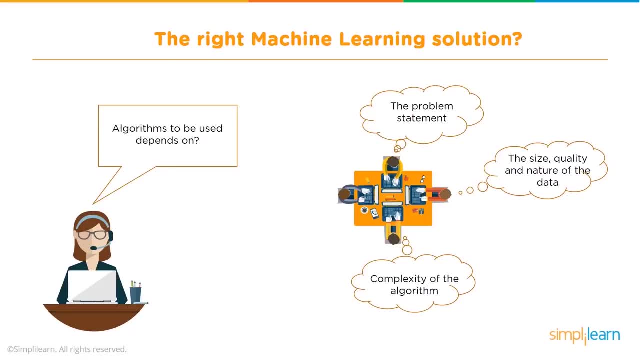 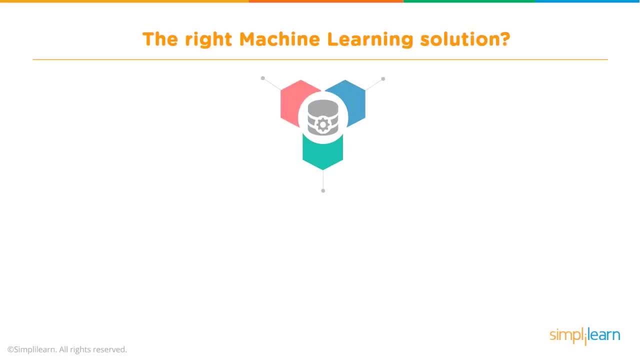 by using reinforcement, But that would be very, very difficult and time consuming. unlike supervised learning, Algorithms are not types of machine learning. In the most simplest language, they are methods of solving a particular problem. The first kind of method is classification, which falls under supervised learning. 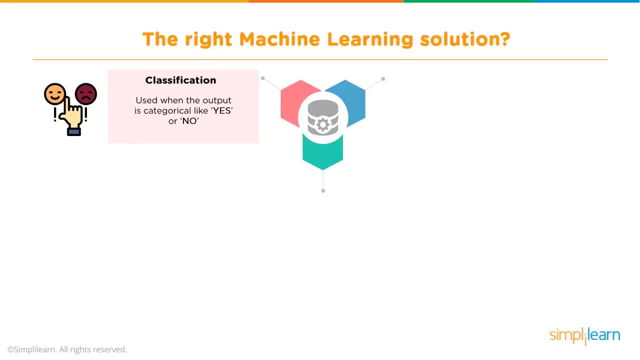 Classification is used. when the output you are looking for is a yes or a no, or in the form A or B or true or false, Like if a shopkeeper wants to predict the future stock market prices, you can use the classification algorithm. 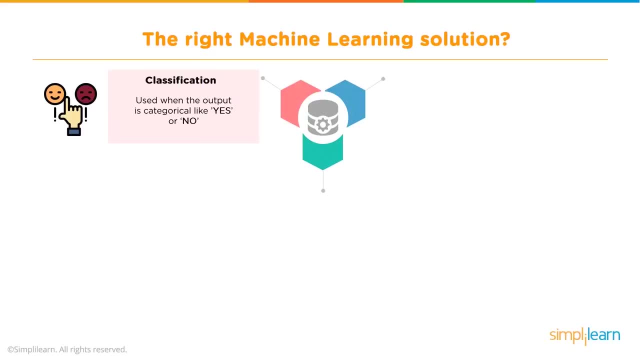 If the shopkeeper wants to predict if a particular customer will come back to his shop or not, he will use a classification algorithm. The algorithms that fall under classification are decision, tree, knife base, random forest, logistic regression and KNN. The next kind is regression. 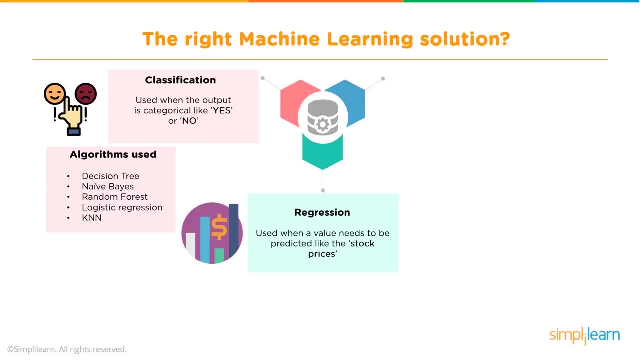 This kind of a method is used when the predicted data is numerical in nature, Like if the shopkeeper wants to predict the price of a product based on its demand. it would go for regression. The last method is clustering. Clustering is a kind of unsupervised learning again. 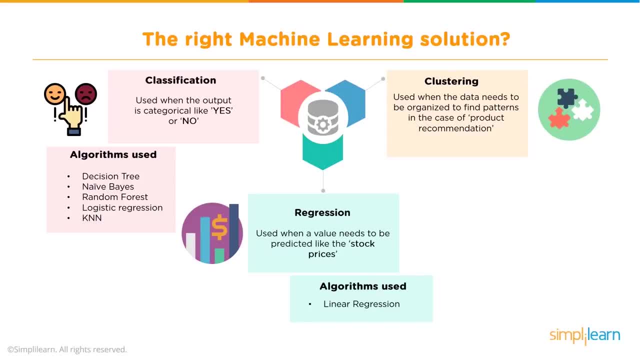 It is used when the data needs to be organized. Most of the recommendation systems used by Flipkart, Amazon, etc. make use of clustering. Another major application of it is in search engines. The search engines study your old search history to figure out your preferences and provide. 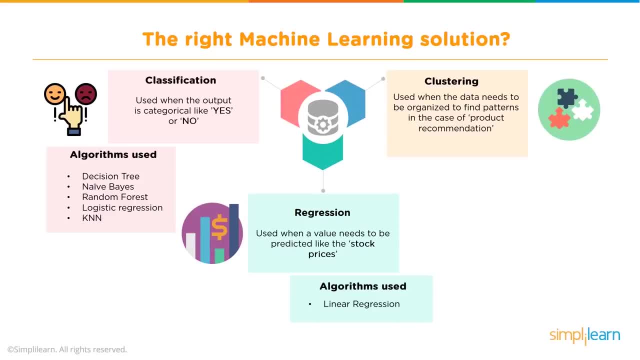 Clustering is a kind of unsupervised learning. again, It is used when the data needs to be organized. Most of the recommendation systems used by Flipkart, Amazon, etc. make use of clustering. Another major application of it is in search engines. 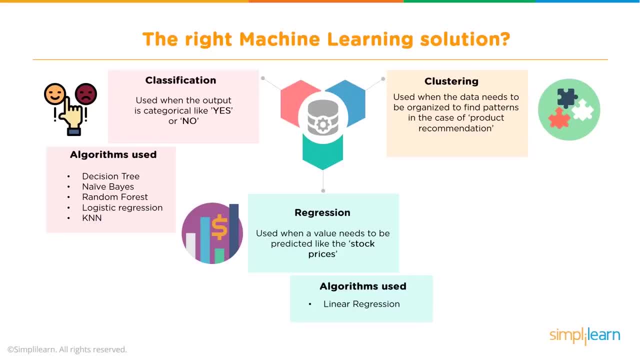 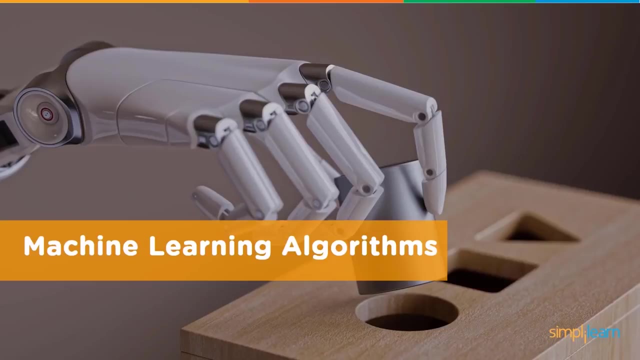 The search engines study your old search history to figure out your preferences and provide you the best search results. One of the algorithms that fall under clustering is K-means. Now that we know the various algorithms, let's look into four key algorithms that are used widely. 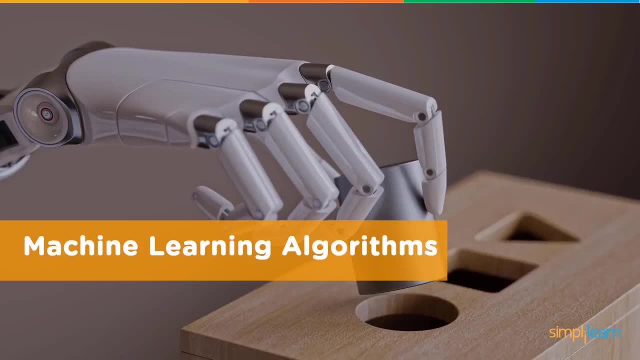 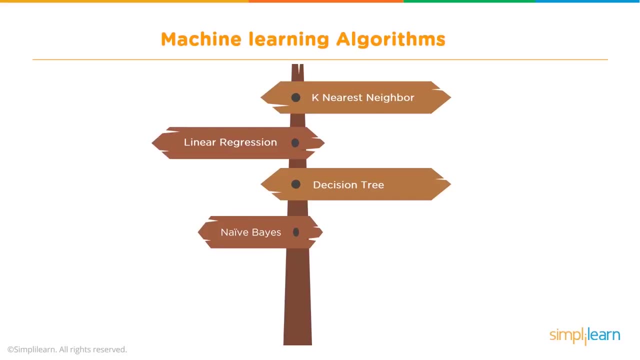 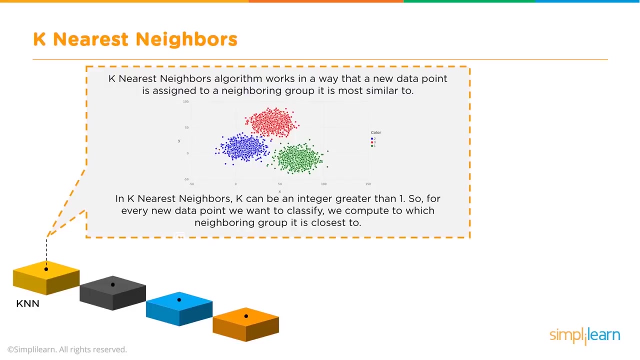 We will understand them with very simple examples. The four algorithms that we will try to understand are K-nearest neighbor, linear regression, decision tree and knife base. Let's start with our first machine learning solution: K-nearest neighbor. K-nearest neighbor is again a kind of a classification algorithm. 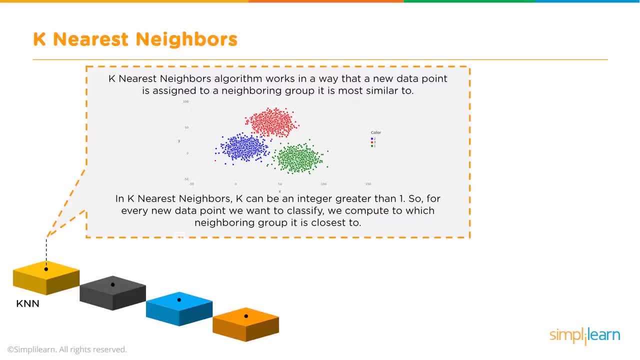 As you can see on the screen, the similar data points form clusters: The blue one, the red one and the green one. There are three different clusters. Now, if we get a new and unknown data point, it is classified based on the cluster closest to it or the most similar to it. 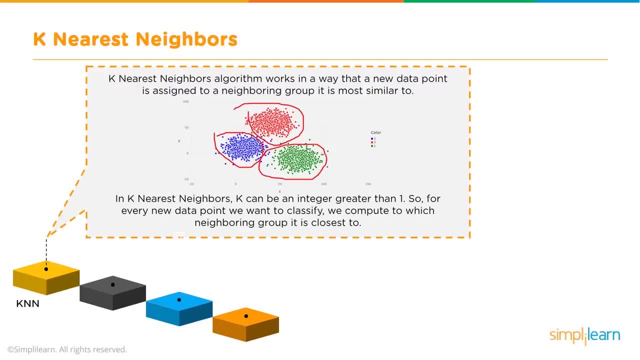 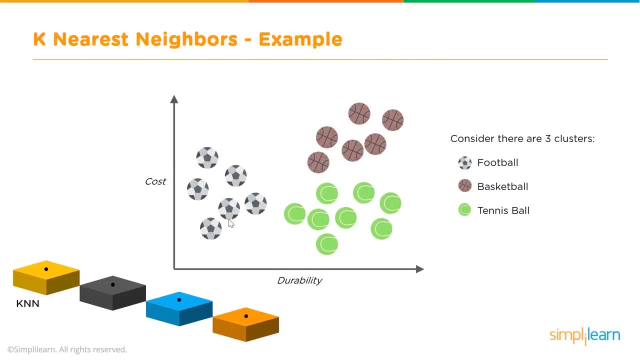 K in KNN is the number of nearest neighboring data points we wish to compare the unknown data with. Let's make it clear with an example. Let's say we have three clusters in a cost to durability graph. First cluster is of footballs. 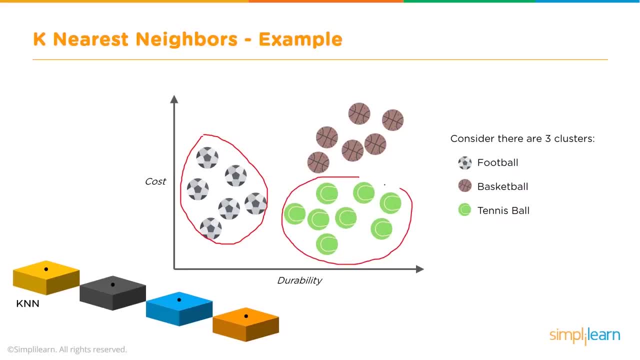 Second one is of tennis balls And the third one is of basketballs. From the graph we can say that the cost of footballs is high and the durability is less. The cost of tennis balls is very less, but the durability is high. 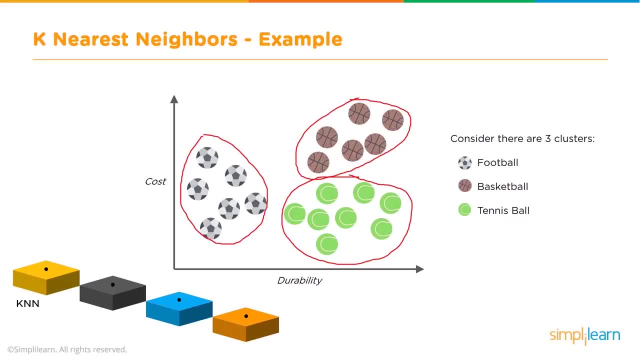 And the cost of basketballs is as high as the durability. Now let's say we have an unknown data point. We have a black spot which can be one kind of the balls, but we don't know what kind it is. So what we'll do? we'll try to classify this using KNN. 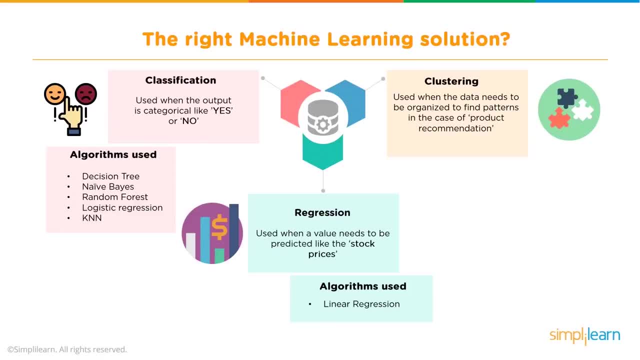 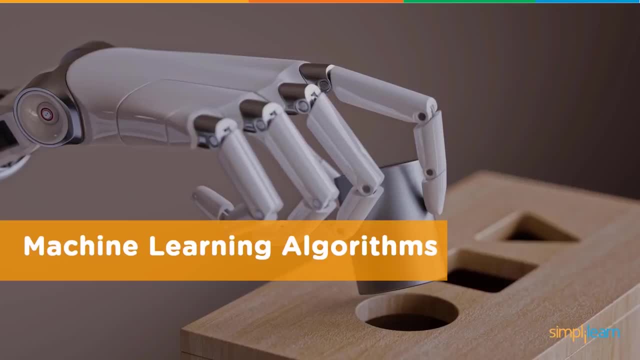 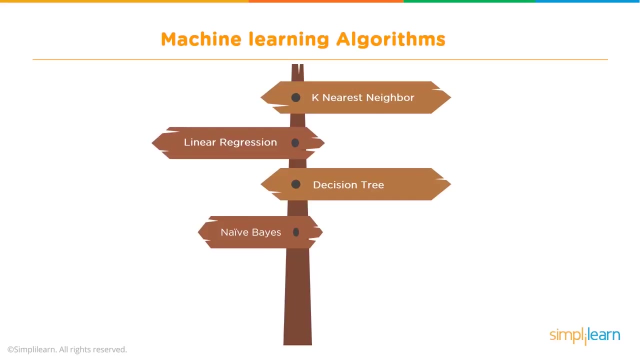 you the best search results. 1. The first algorithm that falls under clustering is K-means. Now that we know the various algorithms, let's look into four key algorithms that are used widely. We will understand them with very simple examples. The four algorithms that we will try to understand are: K-nearest neighbor, linear regression. 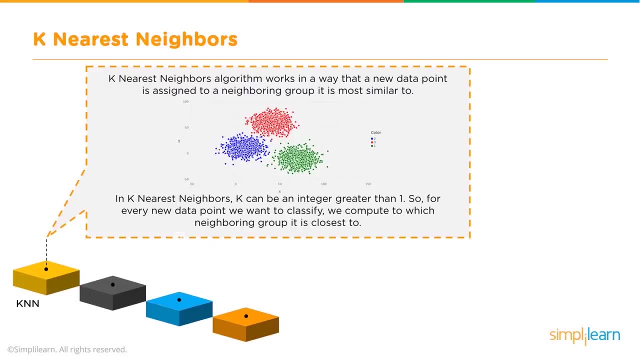 decision tree and knife base. Let's start with our first machine learning solution: K-nearest neighbor 2.. K-nearest neighbor is again a kind of classification algorithm. As you can see on the screen, the similar data points form clusters. 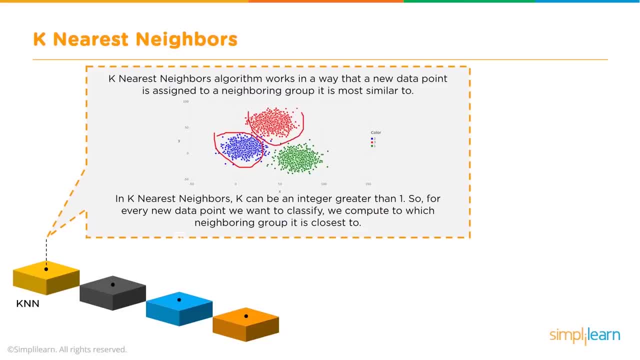 The blue one, the red one and the green one. There are three different clusters. Now if we get a new and unknown data point, it is classified based on the cluster closest to it or the most similar to it. K in KNN is the number of nearest neighboring data points. we wish to compare the unknown. 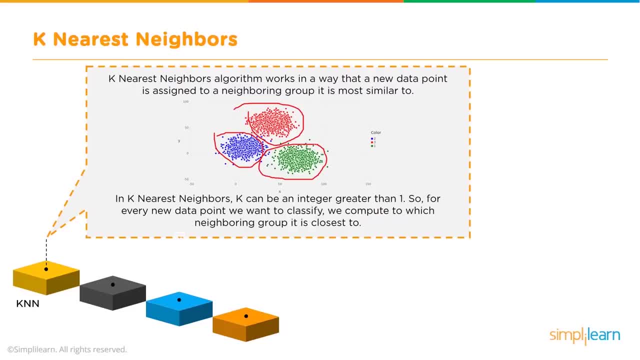 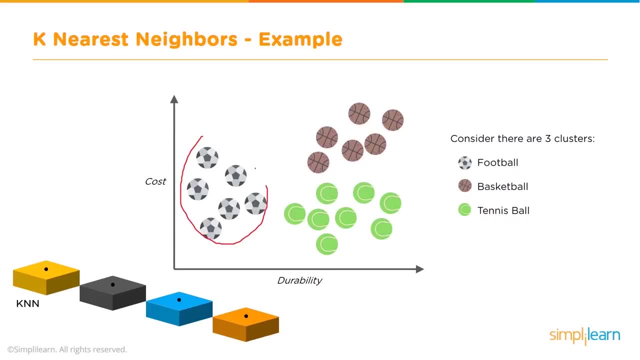 data with. Let's make it clear with an example. Let's say we have three clusters in a cost to durability graph. First cluster is of footballs, Second one is of tennis balls And the third one is of basketballs. From the graph we can say that the cost of footballs is high and the durability is less. 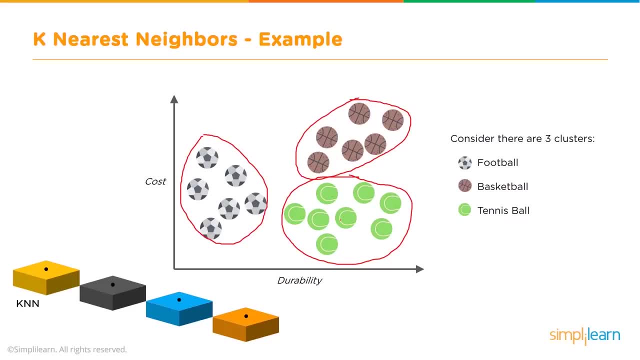 The cost of tennis balls is very less, but the durability is high And the cost of basketballs is as high as the durability. Now let's say we have an unknown data point. We have a black spot which can be one kind of the balls, but we don't know what kind. 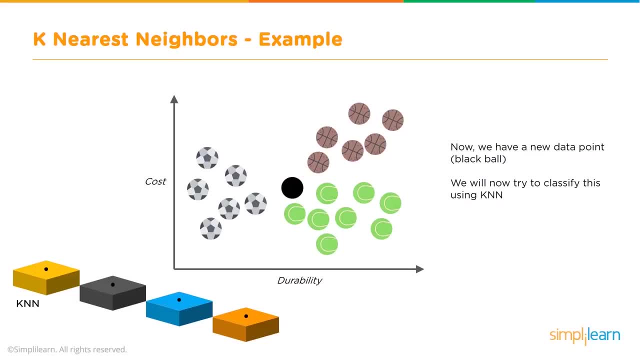 it is So what we'll do. we'll try to classify this using KNN. So if we take, K is equal to 5, we draw a circle keeping the unknown data point at the center And we make sure that we have five balls inside that circle. 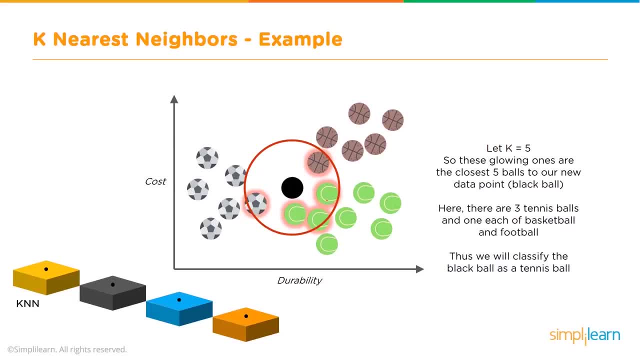 In this case we have a football, A basketball And three tennis balls. Since we have the highest number of tennis balls inside the circle, the classified ball would be a tennis ball. So that's how K-nearest neighbor classification is done. 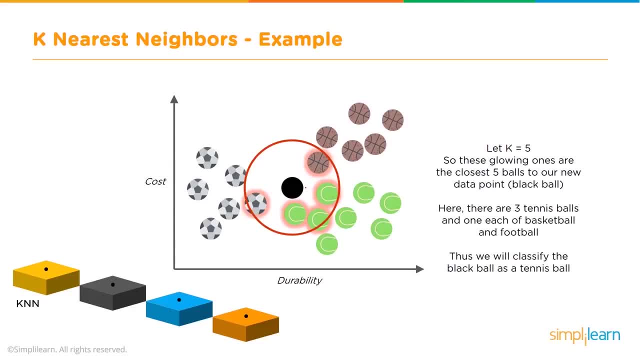 So, if we take, K is equal to 5, we draw a circle keeping the unknown data point at the center And we make sure that we have 5 balls inside that circle. In this case, we have a football, a basketball and three tennis balls. 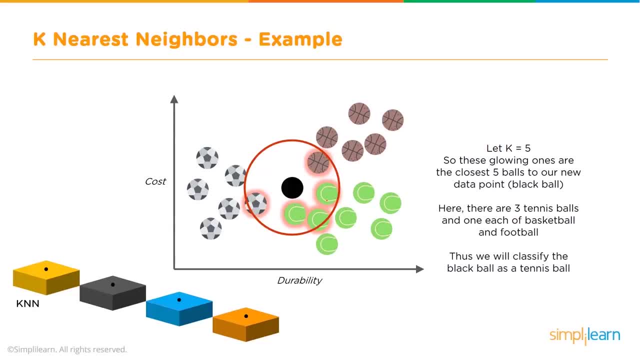 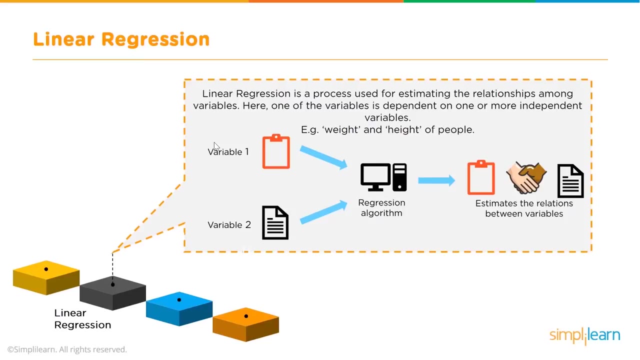 Now, since we have the highest number of tennis balls inside the circle, the classified ball would be a tennis ball. So that's how K-nearest neighbor classification is done. Linear regression is again a type of supervised learning algorithm. This algorithm is used to establish linear relationship between variables, one of which would be dependent and the other one would be independent. 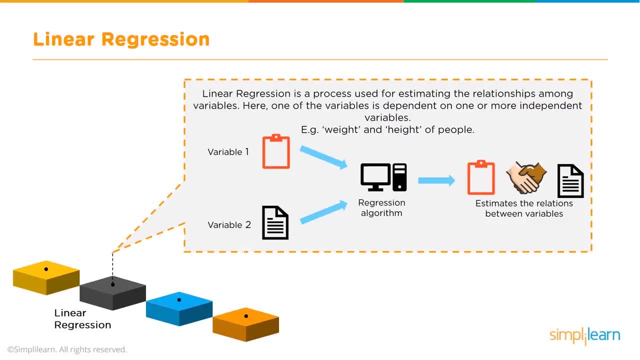 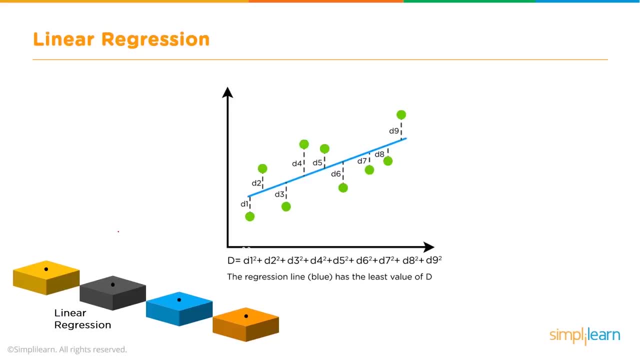 Like if we want to predict the weight of a person based on his height, weight would be the dependent variable and height would be independent. Let's have a look at it through an example. Let's say we have a graph here showing a relationship between height and weight of a person. 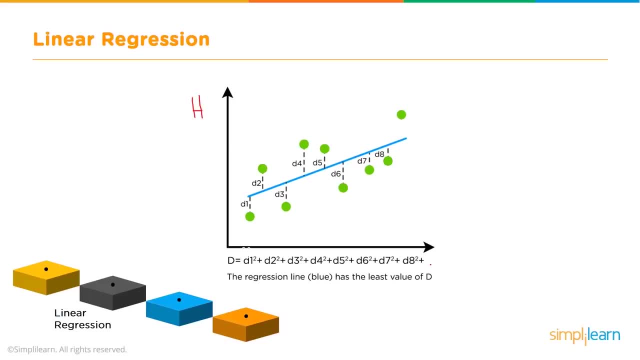 Let's put the y-axis as h and the x-axis as weight. So the green dots are the various data points. These green dots are the data points And d is the mean squared error. that is, the perpendicular distances from the line to the data points are the error values. 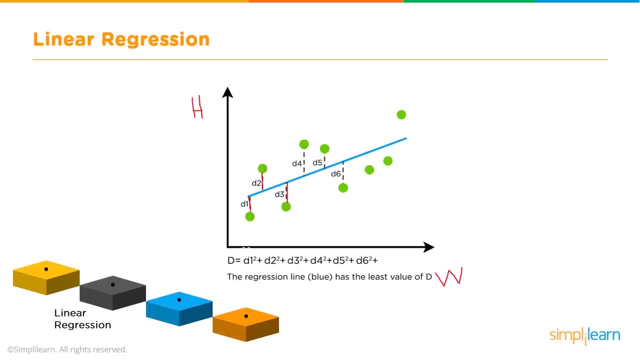 This error tells us how much the predicted values vary from the original value. Let's ignore this blue line for a while. So let's say if this is our regression line. You can see the distance from all the data points from this line is very high. 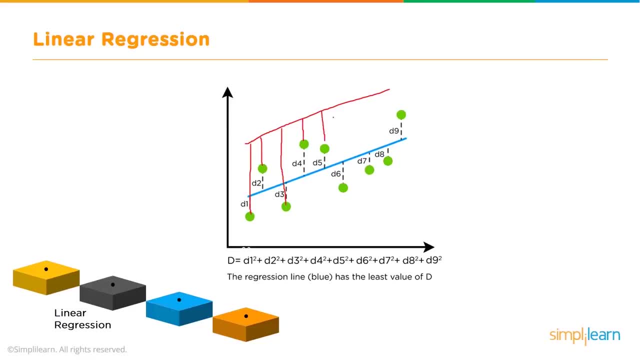 So if we take this line as a regression line, the error in the prediction will be too high. So in this case the model will not be able to give us a good prediction. Let's say we draw another regression line like this. Even in this case you can see that the perpendicular distance of the data points from the line is very high. 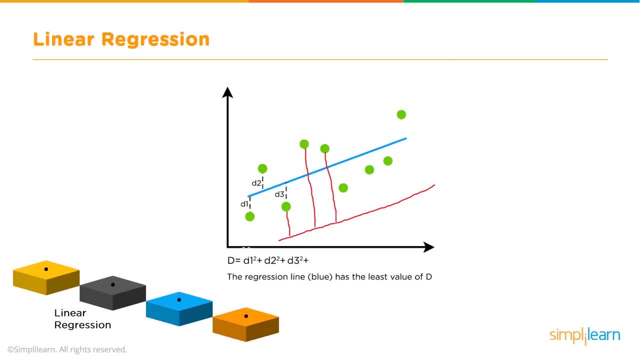 So the error value will still come as high as the last one. So this model will also not be able to give us a good prediction. So what to do? So, finally, we draw a line, which is this blue line. So here we can see that the distance of the data points from the line is very less. 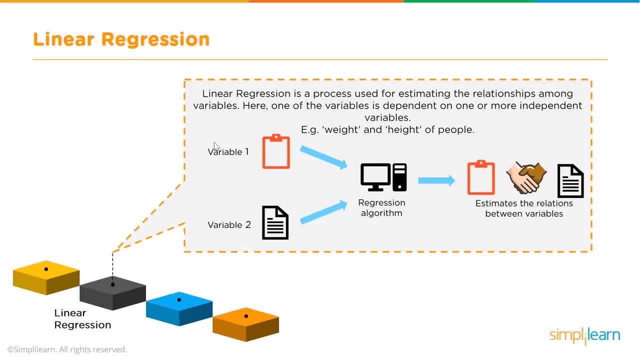 Linear regression is again a type of supervised learning algorithm. This algorithm is used to establish linear relationship between variables, one of which would be dependent and the other one would be independent, Like if we want to predict the world, To predict the weight of a person based on his height, weight would be the dependent. 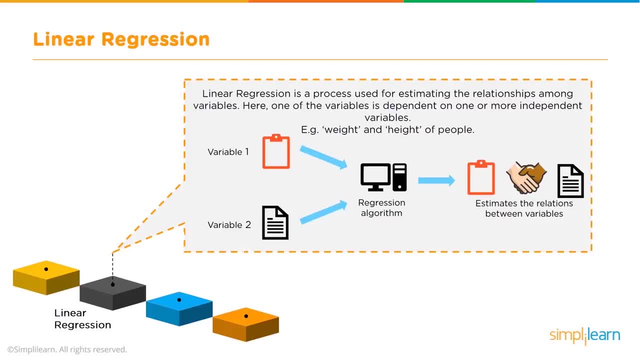 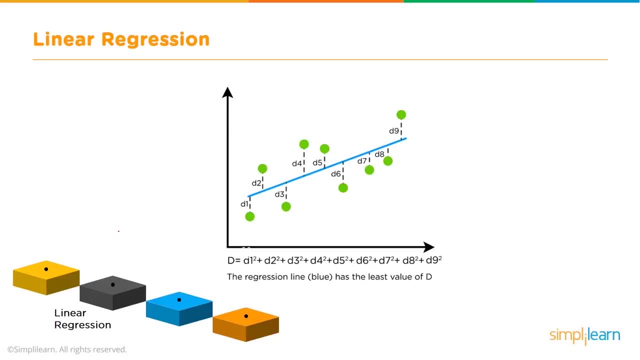 variable and height would be independent. Let's have a look at it through an example. Let's say we have a graph here showing a relationship between height and weight of a person. Let's put the y-axis as h and the x-axis as weight. 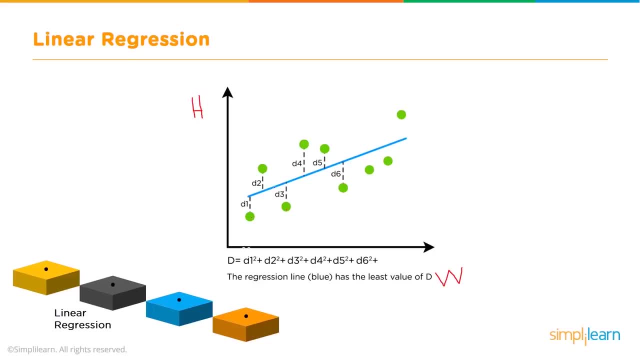 So the green dots are the various data points. These green dots are the data points. So the green dots are the various data points. These green dots are the data points. And d is the mean squared error. that is the perpendicular distances from the line to the. 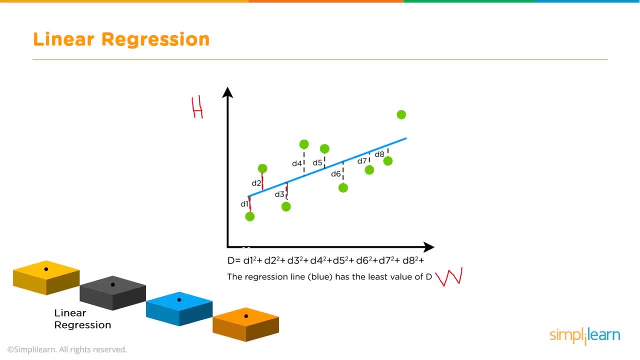 data points are the error values. This error tells us how much the predicted values vary from the original value. Let's ignore this blue line for a while. So let's say: if this is our regression line, you can see the distance from all the data. 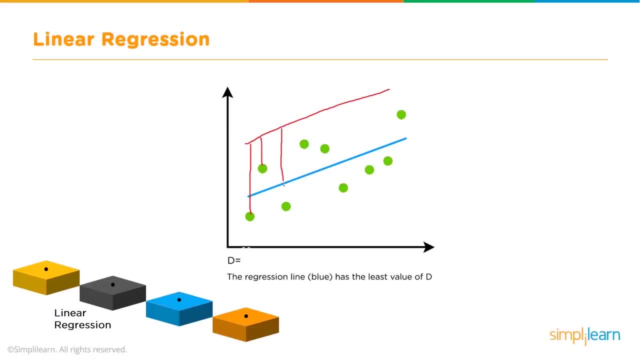 points from this line is 1.5.. It's very high. So if we take this line as a regression line, the error in the prediction will be too high. So in this case the model will not be able to give us a good prediction. 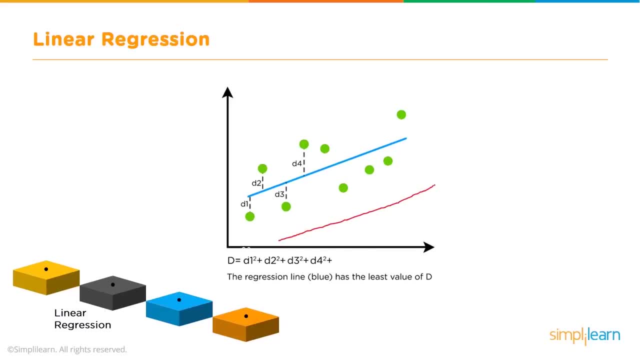 Let's say we draw another regression line like this: Even in this case you can see that the perpendicular distance of the data points from the line is very high, So the error value will still come as high as the last one. So this model will also not be able to give us a good prediction. 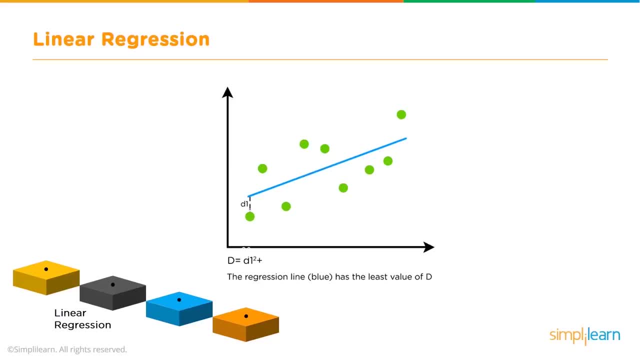 So what to do? So finally, we draw a line, which is this blue line. So here we can see that the distance of the data points from the line is very less relative to the other two lines we drew, So the value of d for this line will be very less. 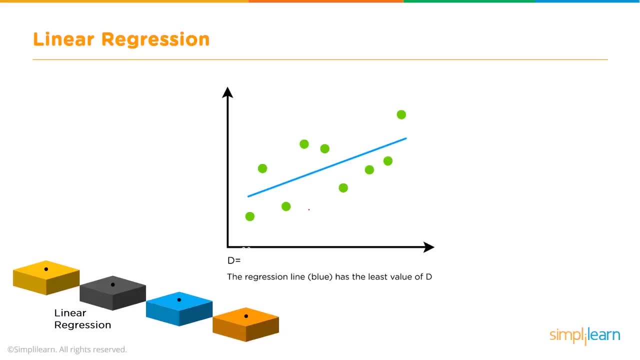 So in this case, if we take any value on the x-axis, the corresponding value on the x-axis, the corresponding value on the x-axis will be very less. So in this case, if we take any value on the x-axis, the corresponding value on the 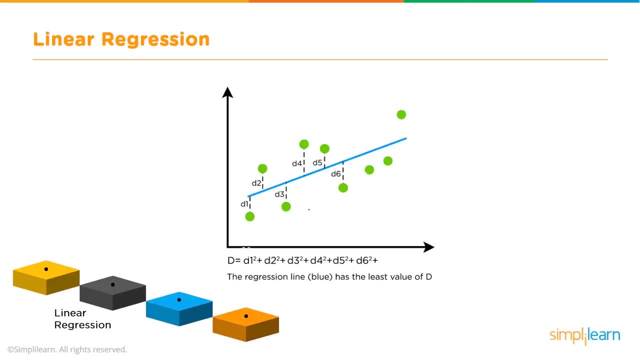 Relative to the other two lines we drew. So the value of d for this line will be very less. So in this case, if we take any value on the x-axis, the corresponding value on the y-axis will be our prediction And, given the fact that the d is very low, our prediction should be good also. 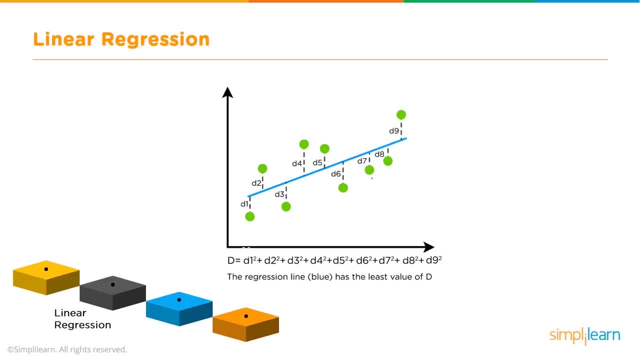 This is how regression works. We draw a line, a regression line that is in such a way that the value of d is the least, Eventually giving us good predictions. This algorithm, that is, decision tree, is a kind of an algorithm you can very strongly relate to. 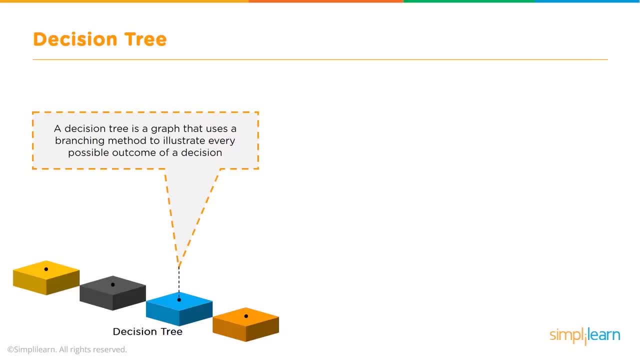 It uses a kind of a branching method to realize the problem and make decisions based on the conditions. Let's take this graph as an example. Imagine yourself sitting at home getting bored. You feel like going for a swim. What you do is you check if it's sunny outside. 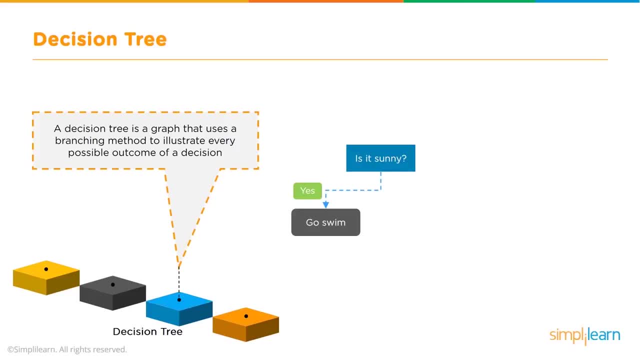 So that's your first condition. If the answer to that condition is yes, you go for a swim. If it's not sunny, then the next question you would ask yourself is if it's raining outside. So that's condition number two. If it's actually raining, you cancel the plan and stay indoors. 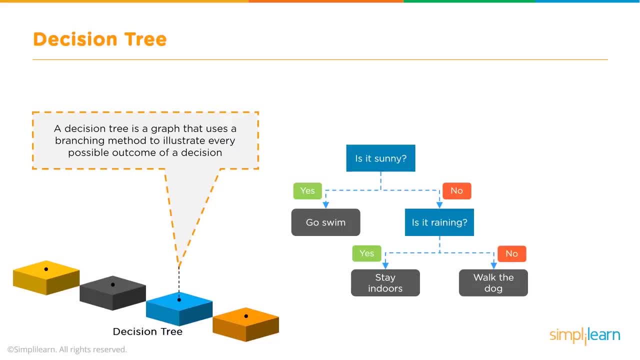 If it's not raining, then you would probably go outside and have a walk. So that's the final node. That's how decision tree algorithm works. You probably use this every day. It realizes the problem and then takes the decisions based on the answers to every conditions. 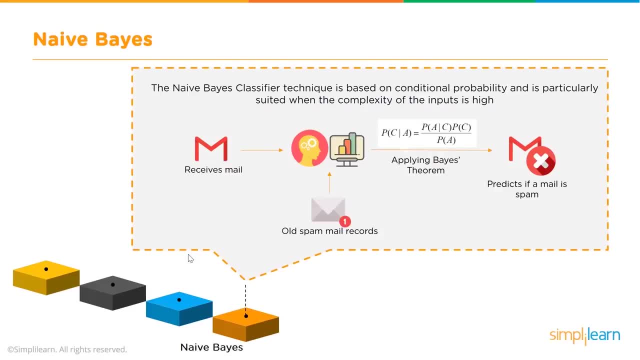 Naib's algorithm is mostly used in cases where a prediction needs to be done on a very large dataset. It makes use of conditional probability. Conditional probability is the probability of an event, say A, happening given that another event B has already happened. This algorithm is most commonly used in filtering spam mails in your email account. 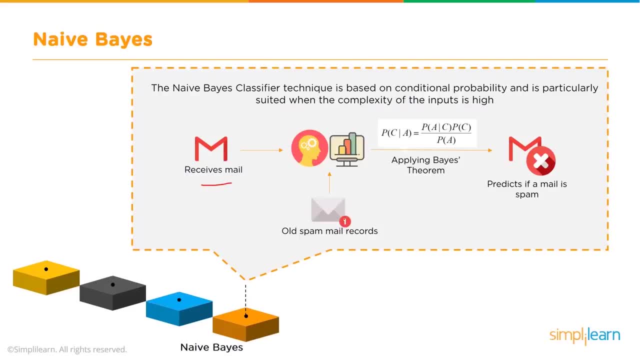 Let's say you receive a mail. The model goes through your old spam mail records, Then it uses Bayes theorem to predict if the present mail is a spam mail or not. So PC of A is the probability of event C occurring when A has already occurred. 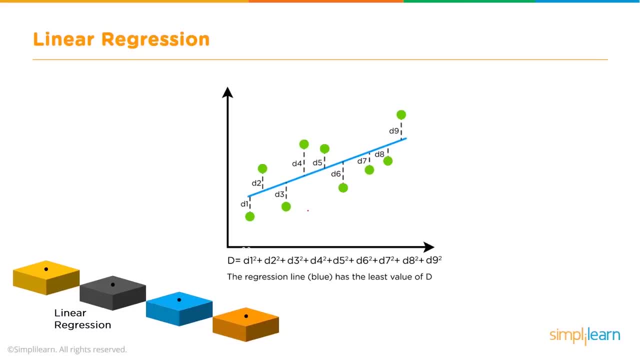 y-axis will be our prediction And, given the fact that the d is very low, our prediction should be good. also, This is how regression works. We draw a line, a regression line, that is in such a way that the value of d is the least. 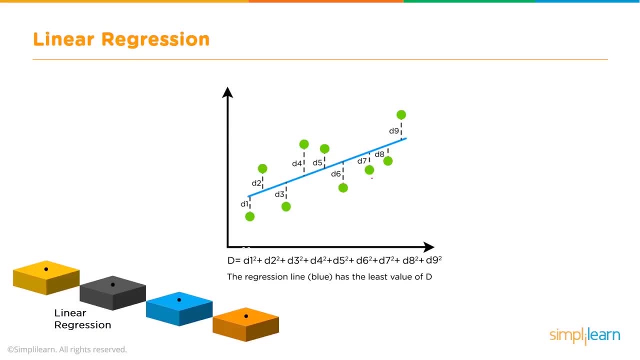 eventually giving us good predictions. This algorithm, that is, decision tree, is a kind of an algorithm you can very strongly relate to. It uses a kind of a branching method to realize the problem and make decisions based on the conditions. Let's take this graph as an example. 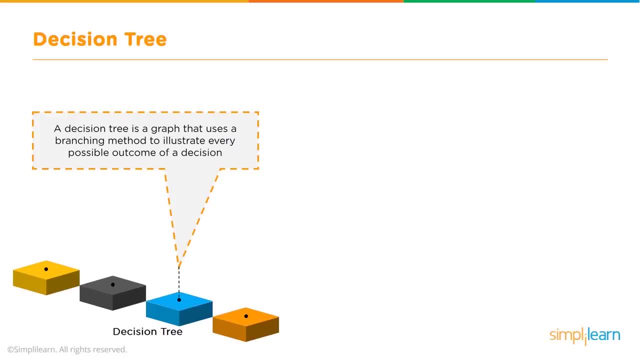 Imagine yourself sitting at home getting bored. You feel like going for a swim. What you do is you check if it's sunny outside. So that's your first condition. If the answer to that condition is yes, you go for a swim. If it's not sunny, then the next question you would ask yourself is if it's raining. 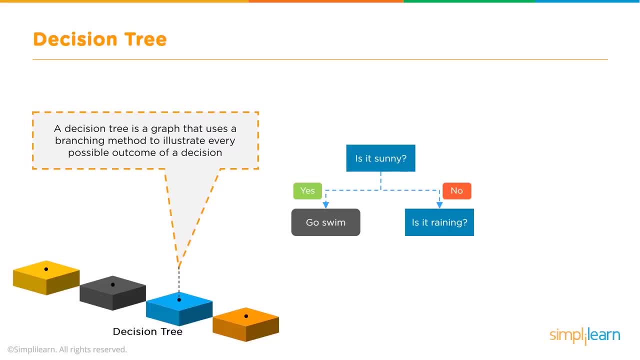 outside. So that's condition number two. If it's actually raining, you cancel the plan and stay indoors. So that's condition number two. So that's condition number three. If it's not raining, then you would probably go outside and have a walk. 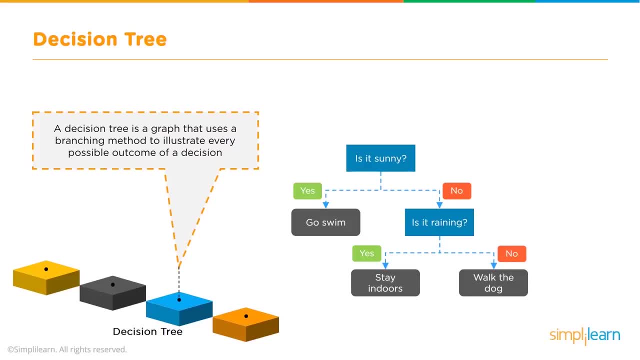 That's the final node. That's how decision tree algorithm works. You probably use this every day. It realizes a problem and then takes the decisions based on the answers to every conditions. Naive Bayes algorithm is mostly used in cases where a prediction needs to be done on a very 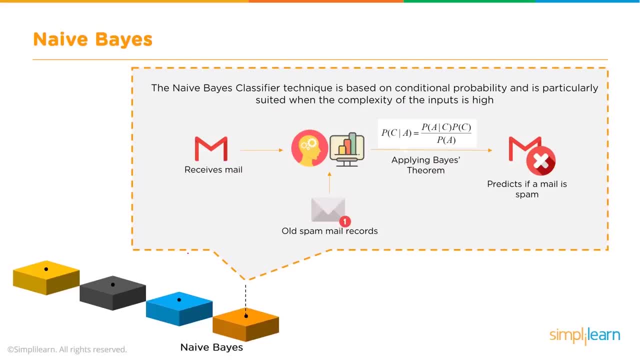 large dataset. It makes use of conditional probability. Conditional probability is the probability of an event. say A, This is the probability of a very large event happening, given that another event B has already happened. This algorithm is most commonly used in filtering spam mails in your email account. 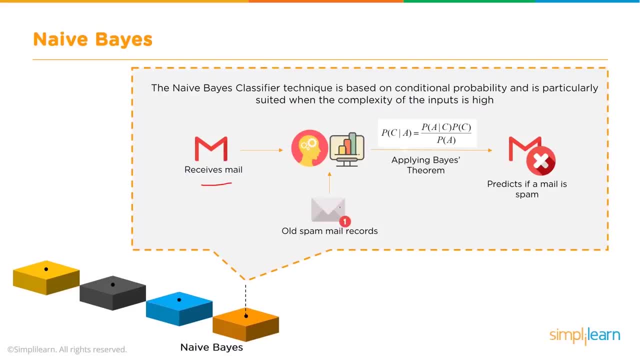 Let's say you receive a mail. The model goes through your old spam mail records, Then it uses Bayes theorem to predict if the present mail is a spam mail or not. So P C of A is the probability of event C occurring when A has already occurred. 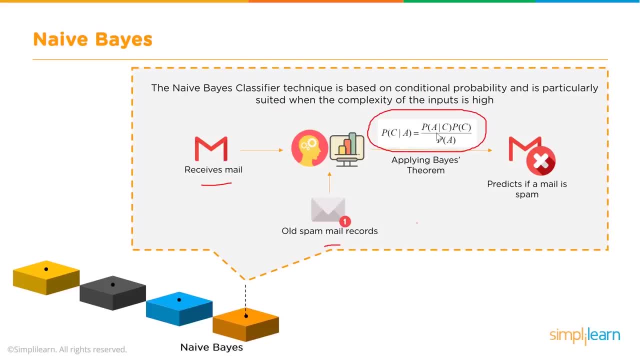 P A of C is the probability of event B occurring when A has already occurred. P A of C is the probability of event B occurring when A has already occurred. is the probability of event A occurring when C has already occurred. and PC is the probability of event C occurring and PA is the probability of event A.